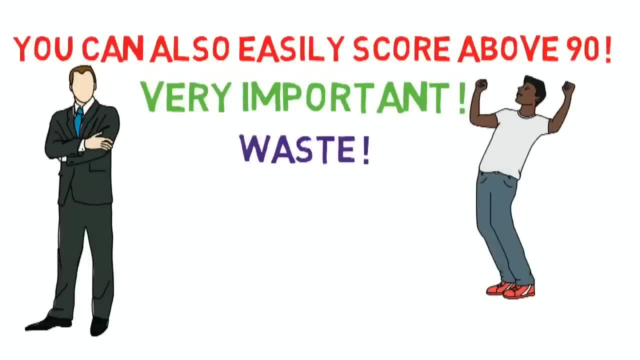 this, you cannot solve any math problem. You have to commit something to yourself. This is very important. Without this, the video will be a waste for you. Now say loudly to yourself that math is easy for me. Yes, say it again. I want to hear you louder, More louder, No matter who is near to you. 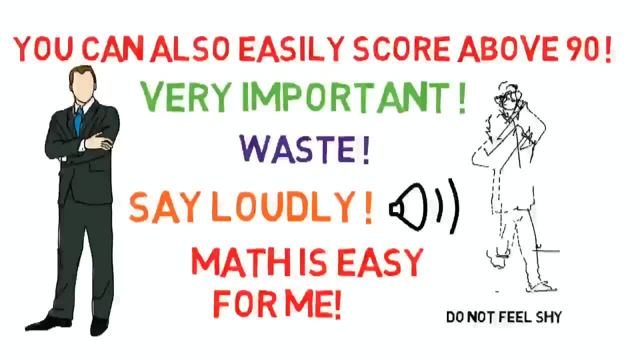 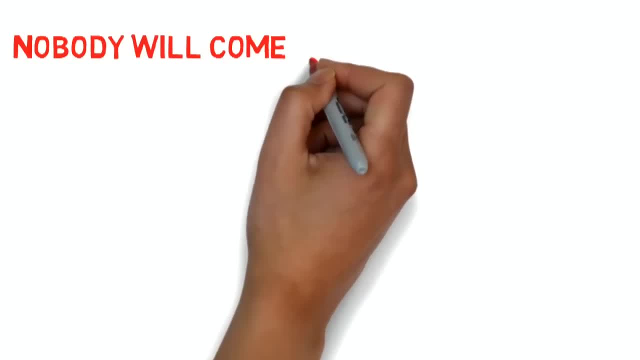 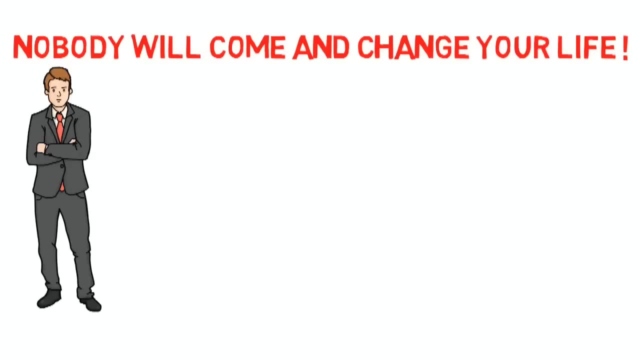 don't feel shy. If you didn't do this, you will go back to your old life, where math is like a demon. So do not care about anybody. Nobody is going to come and change your life. only you can change your life. So say this loudly to yourself: that math is easy for me. 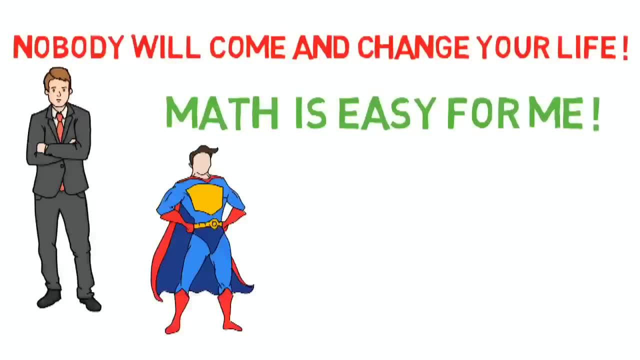 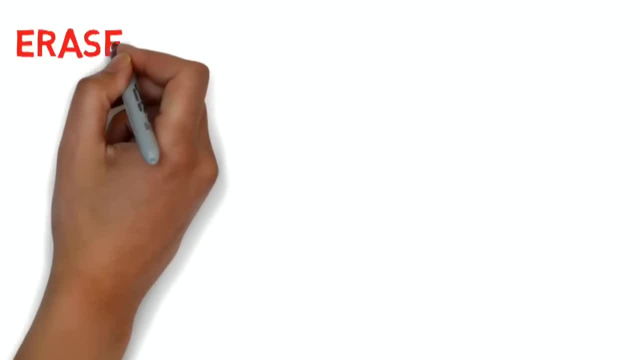 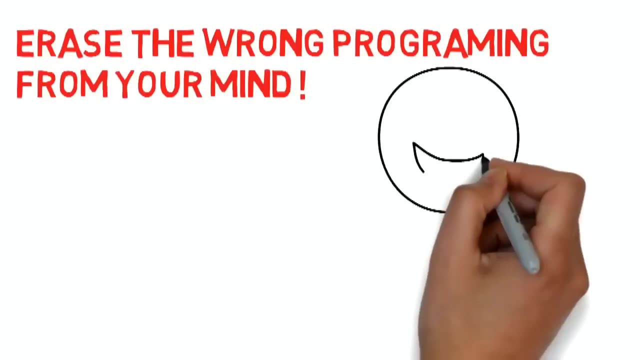 I can solve math easily. Math is a piece of cake for me. Why this is important? I will give you the answer. This is important to take off the wrong mindset, wrong programming in your mind and filling it with positiveness that math is easy for you Once you've. 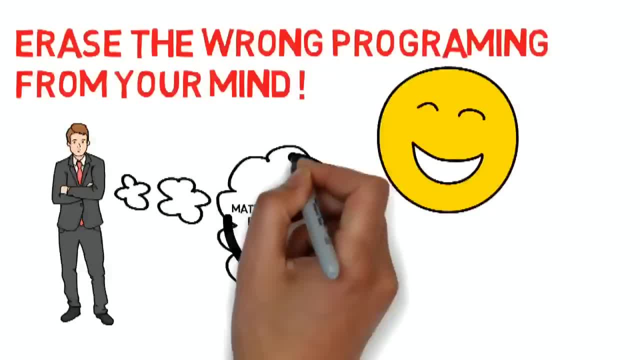 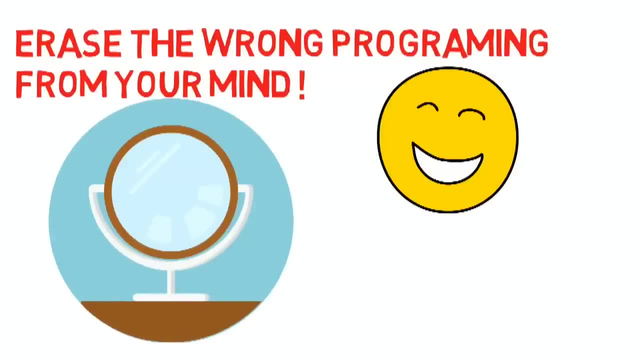 really believe in this, then you are on a right track. If not, pause this video and go in front of a mirror and say this to yourself till you believe this from your within, from your deepest heart: that math is easy for me, Then play this video. I will be always here. So if you are ready, 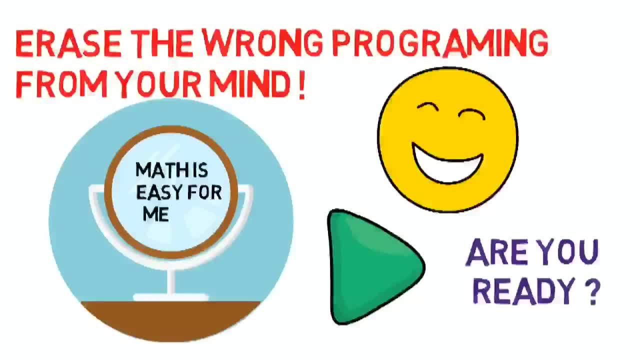 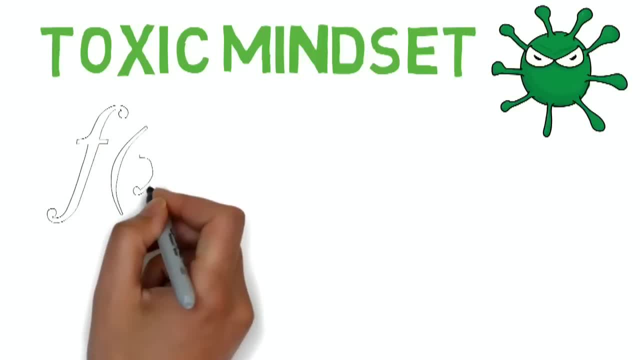 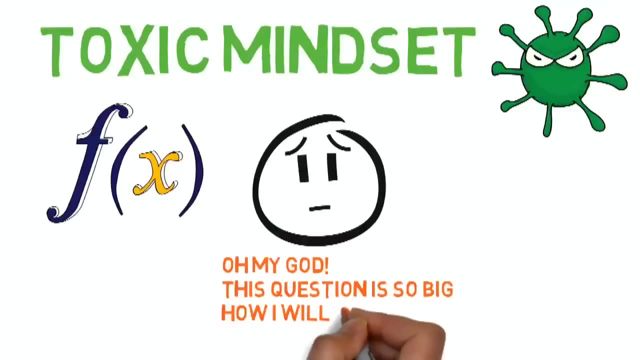 completely ready. let's begin First. I will talk about the most shocking mindset to solve math. Whenever a math problem comes to the most of the people, first they get frightened and say, oh my God, this question is so big. 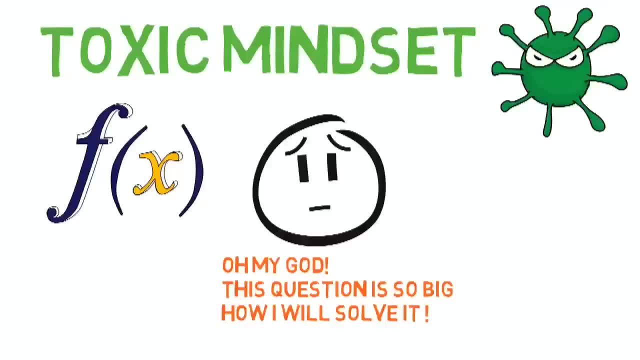 This question is super difficult for me. I can never solve this question. Where is the formula? How I will solve this? It will happen, Blah, blah, blah. But you now, you won't say this because you just changed your mindset. You just changed your mindset. You just changed your mindset. 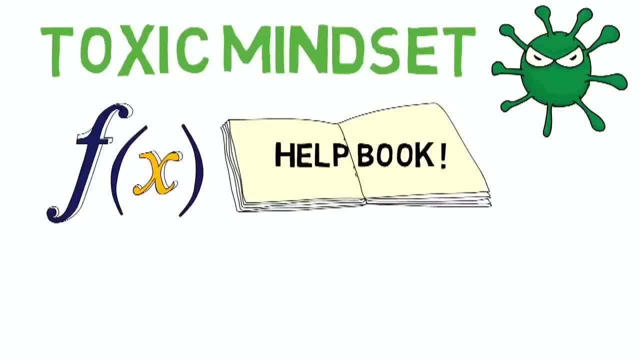 And then suddenly they will open a helpbook in which the solution of that question is already given and they will try to copy the solution from there. After that they will cram the solution from there, And cramming math is the most worst thing you can do. 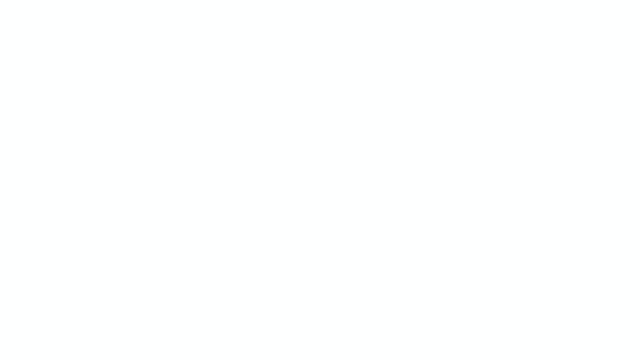 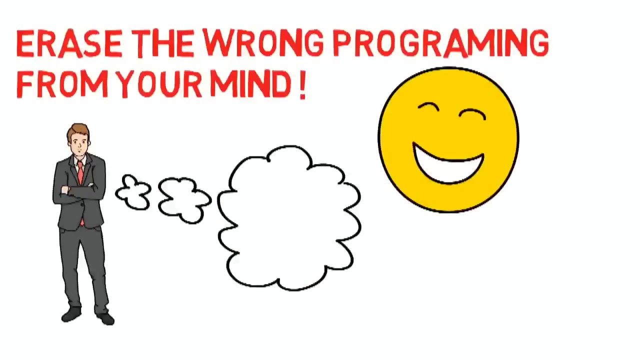 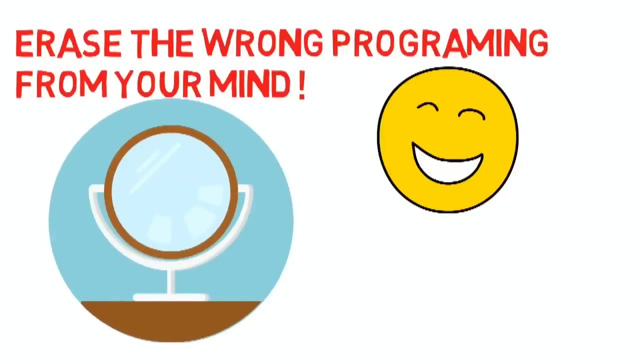 me why this is important. i will give you the answer. this is important to take off the wrong mindset, wrong programming in your mind and filling it with positiveness that math is easy for you. once you really believe in this, then you are on a right track. if not, pause this video and go in front of a mirror and say this to yourself till you believe. 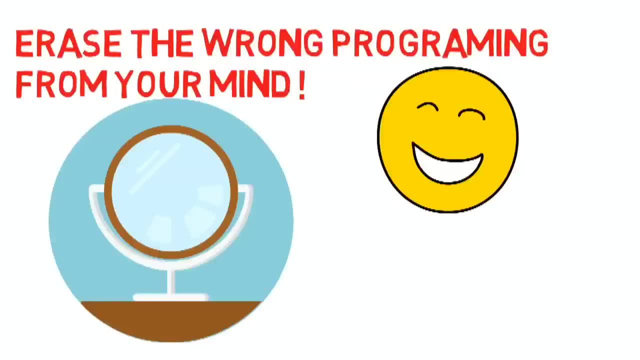 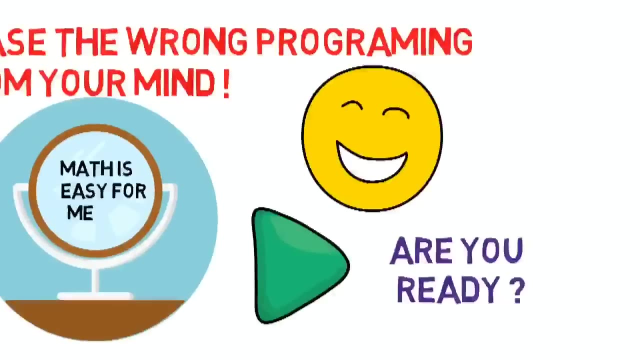 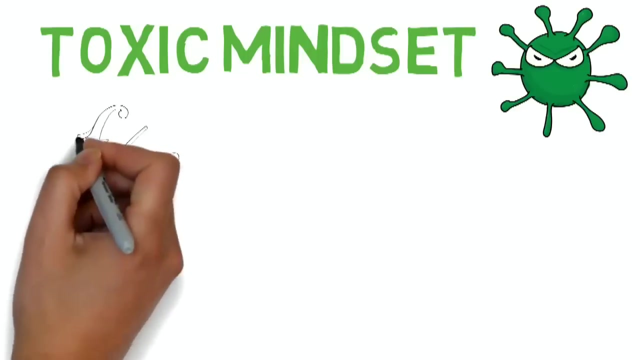 this from your within, from your deepest heart, that math is easy for me. then play this video. i will be always here. so if you are ready, completely ready, let's begin. first i will talk about the most shocking mindset to solve math. whenever a math problem comes to the most of the people, first they get frightened and say, oh my god. 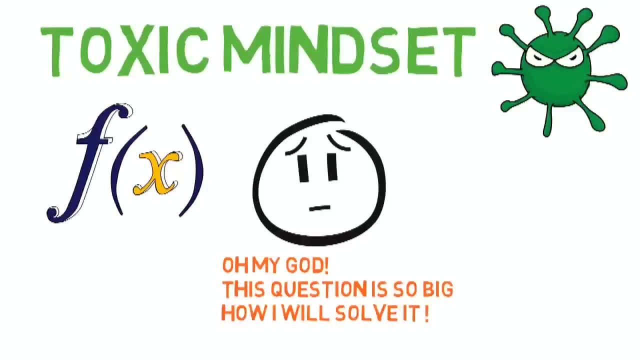 this question is so big. this question is super difficult for me. i can never solve this question. ah, where is the formula how i will solve this? it will happen, blah, blah, blah. but you now, you won't say this because you just changed your mindset. and then suddenly they will open a help book in 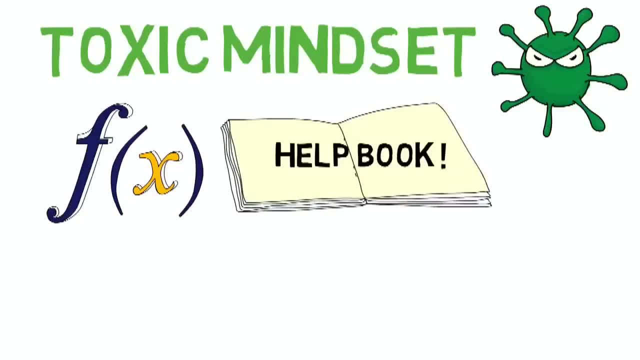 which the solution of that question is already given and they will try to copy the solution from there. after that they will cram the solution from there, and cramming math is the most worst thing you can do about your math. so never cram math. or if they don't find a help book, what will? 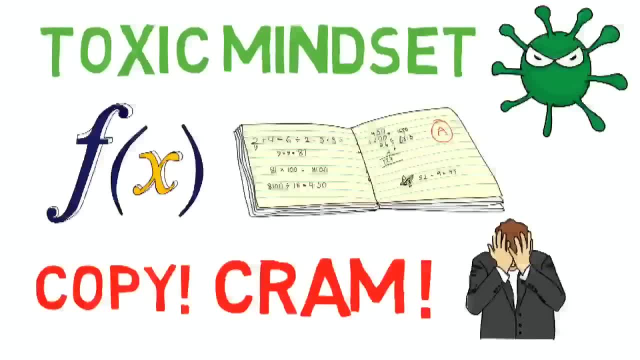 they do, they will find a similar question in which they will say: oh my god, this question is so big, this question is so big, this question is so big. the solution is given and they will try to do the same in that question and it doesn't matter that. 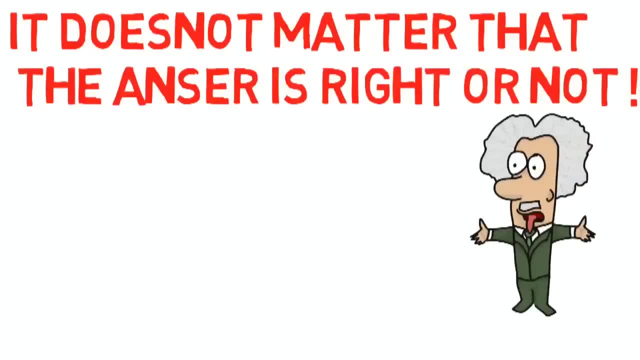 the answer is right or not. if the answer is right, what you have learned from that question? nothing, just cramming, copying, etc. so never do this. this will only make your math difficult for you, and the more you do this, the more you will get stuck in this, because this is like a spider web. so never. 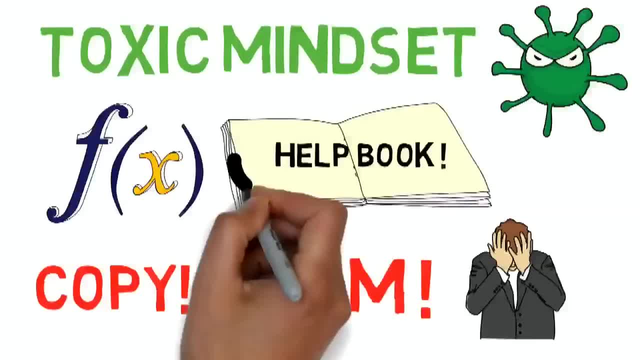 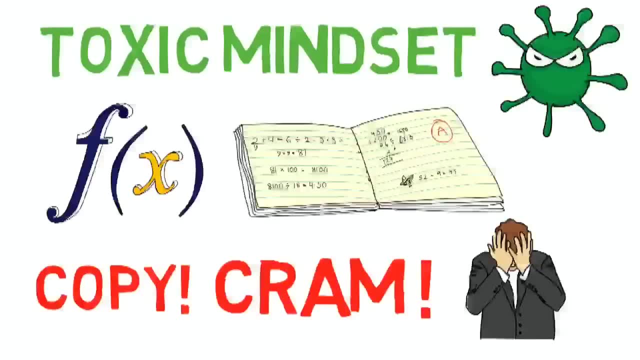 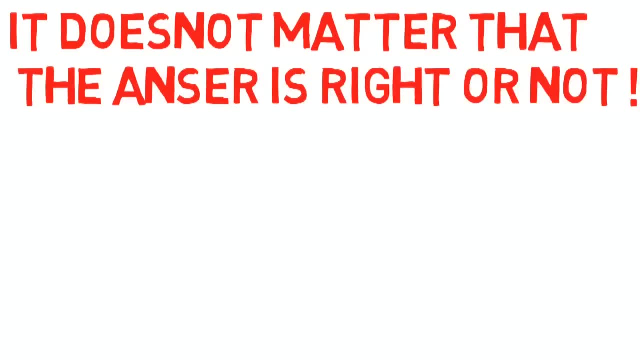 about your math. So never cram math. Or if they don't find a helpbook, what will they do? They will find a similar question in which the solution is given and they will try to do the same in the same in that question, and it doesn't matter that the answer is right or not. if the answer is right, 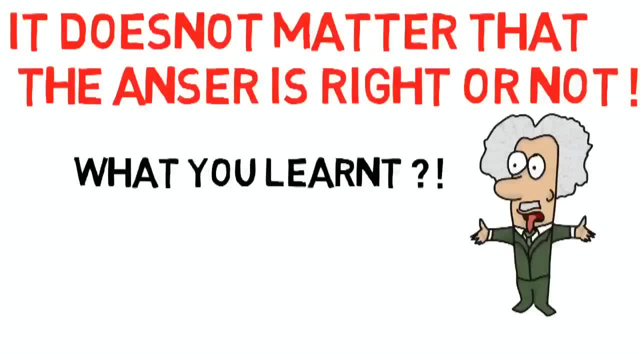 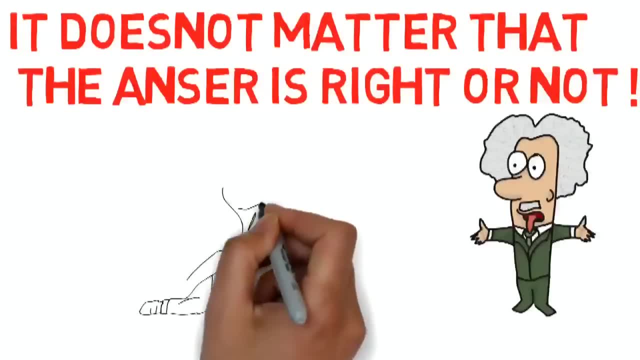 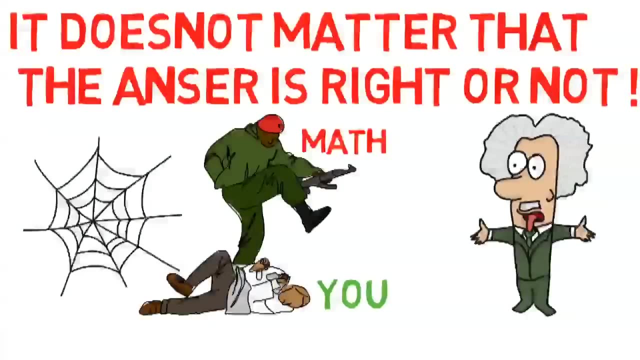 what you have learned from that question? nothing, just cramming, copying, etc. so never do this. this will only make your math difficult for you, and the more you do this, the more you will get stuck in this, because this is like a spider web. so never do this, because the question will only increase. 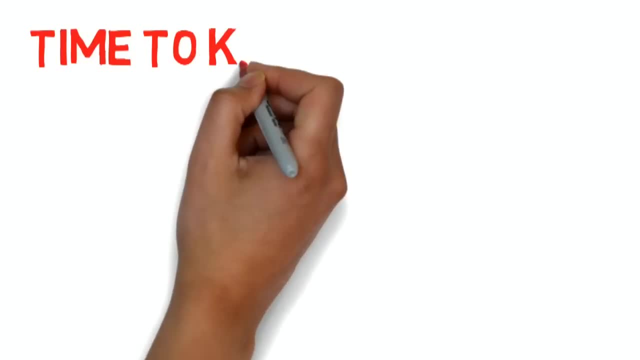 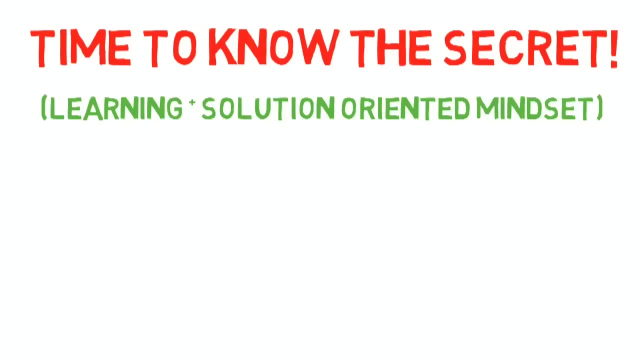 and cramming will not solve this. now the time has come in which i will talk about that mindset. i call it the learning plus solution oriented mindset, in which you focus on learning, trying to learn something from the question, and you focus on finding the solution of that question by focusing. 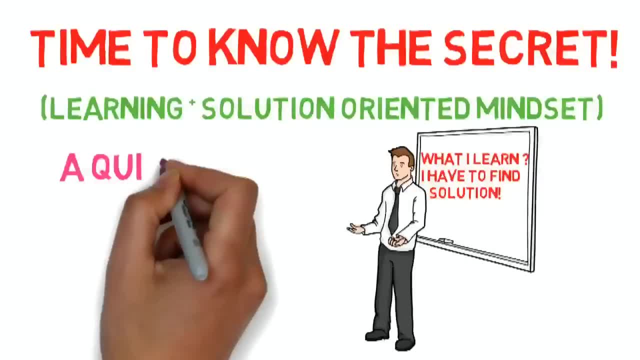 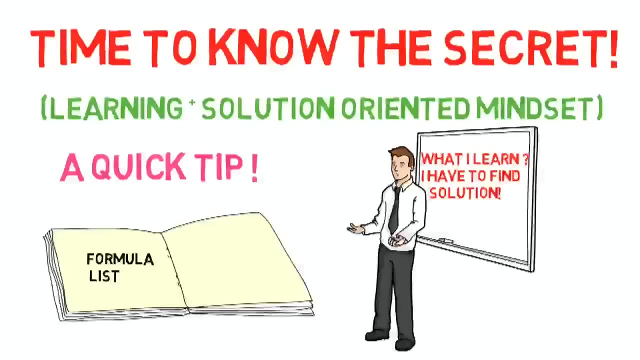 on the problem you have given. first let me give you a tip for solving every math problem. in your math, first make a list of all the formulas which are going to be used in that particular chapter you are going to solve. this is a proven method to solve math problem. if you have a list of formulas which 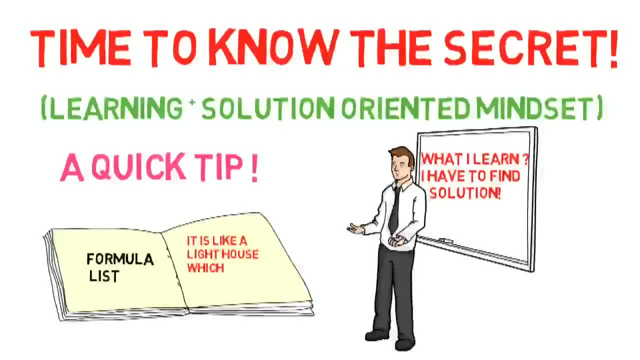 can be used in that problem. this makes math super easy for you. so always before starting a chapter, make a list of all the formulas which are going to be used in that chapter. for example, if you are going to solve trigonometry, then make a list of all the formulas which are going to be used in it. 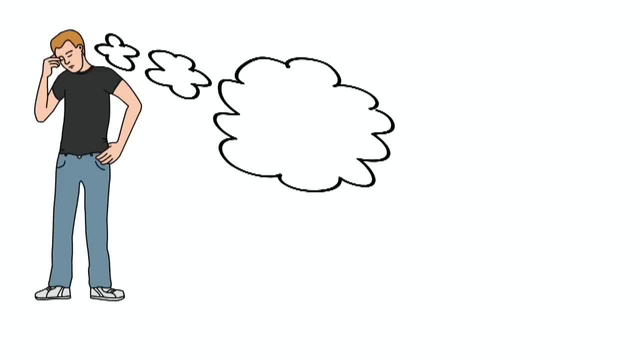 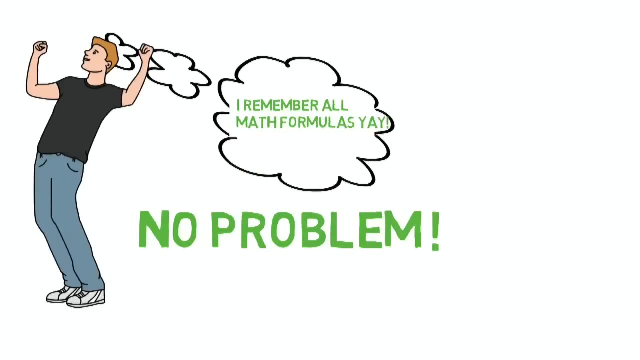 now you will say that i hardly remember any math formula. it is so hard to remember them, i know. but no problem, with this mindset, you will automatically start memorizing all the formulas in your math book without doing any effort. if you practice what i say now, you have a math problem. 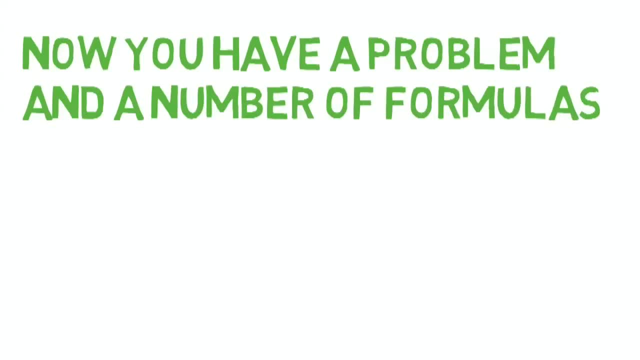 and a number of formulas which are going to be used in that chapter. so make a list of all the formulas to solve that problem. now how will you know which formula is right for the problem? the answer is to read the problem carefully. this is the first and the most important step to solve math problem. 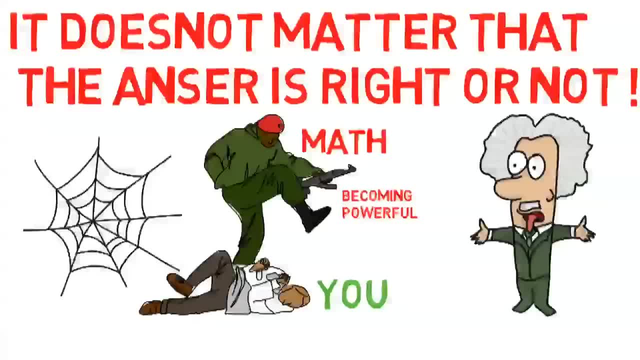 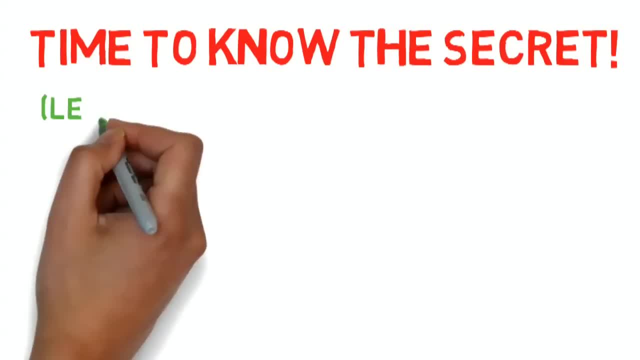 do this because the question will only make you feel like a spider web. so never do this, because only in greens and cramming will not solve this. now the time has come in which i will talk about that mindset. i call it the learning plus solution oriented mindset, in which you focus on learning. 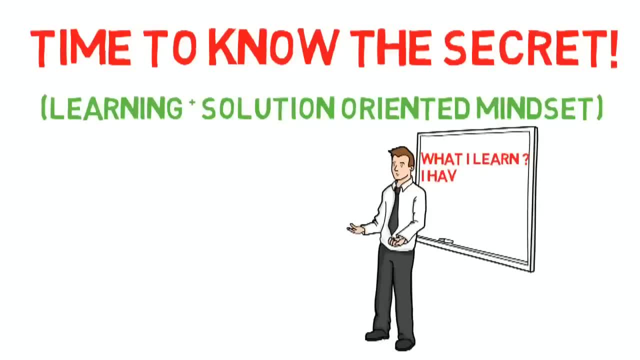 trying to learn something from the question and you focus on finding the solution of that question by focusing on the problem you have given. first, let me give you a tip for solving every math problem in your math books: first make a list of all the formulas which are going to be used in that particular chapter. you. 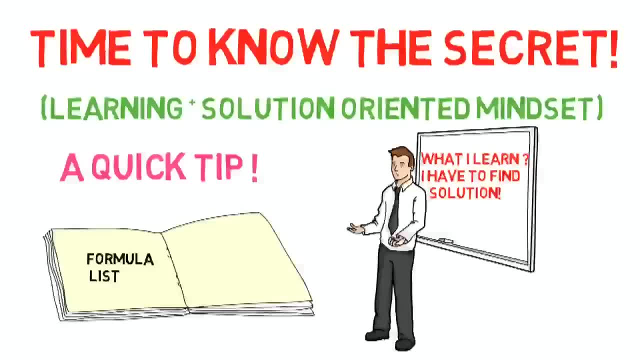 are going to solve. this is a proven method to solve math problem. if you have a list of formulas which can be used in that problem, this makes math super easy for you. so always before starting a chapter, make a list of all the formulas which are going to be used in that chapter. for example, if 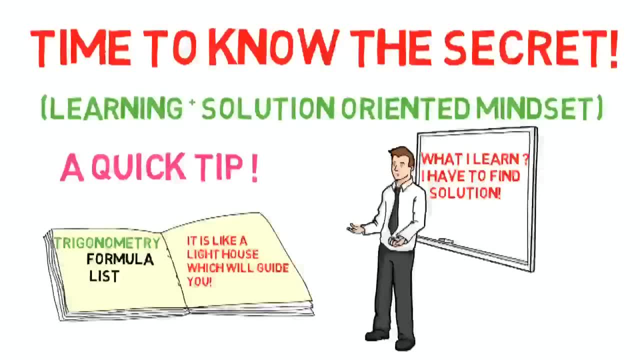 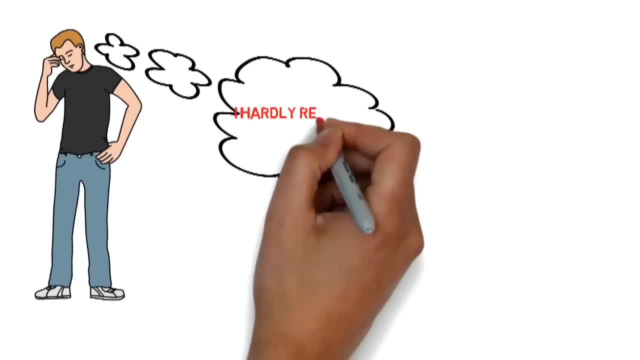 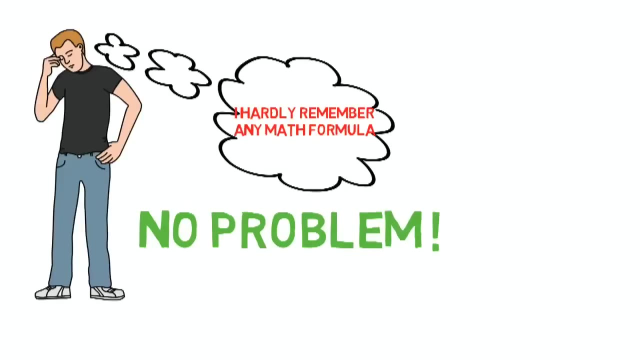 you are going to solve trigonometry, then make a list of all the formulas which are going to be used in it. now you will say that i hardly remember any math formula. it is so hard to remember them, i know. but no problem. with this mindset, you will automatically start memorizing all the formulas in your math book without doing. 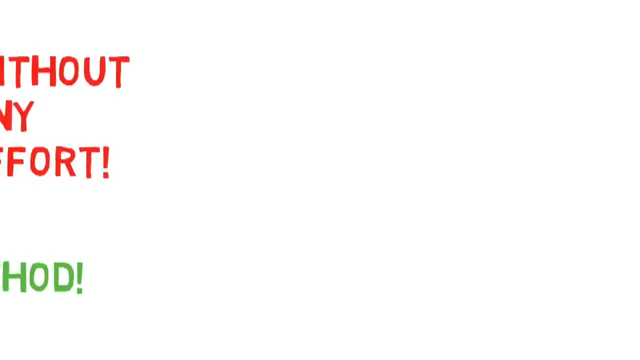 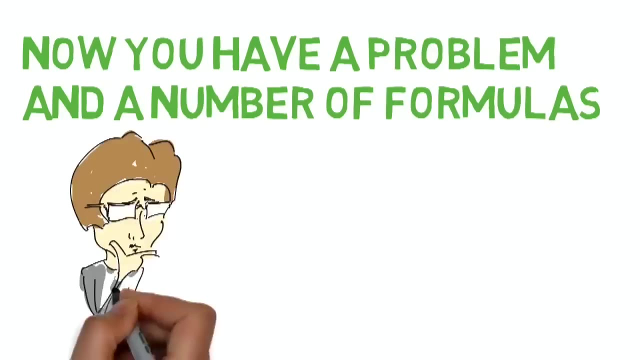 any effort. if you practice what i say now, you have a math problem and a number of formulas to solve that problem. now how will you know which formula is right for the problem? the answer is: to read the problem carefully. this is the first and the most important step to solve math problem. most people 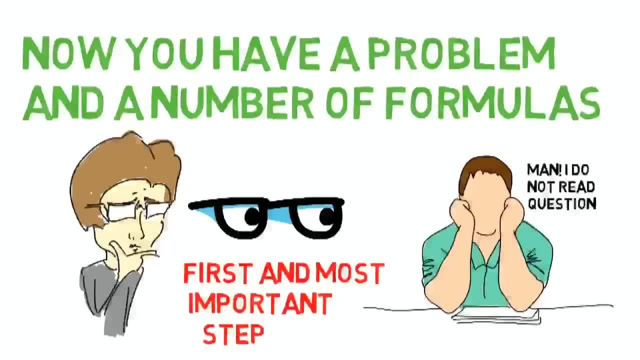 never do this. they never read the problem carefully. they do this. this question is of this chapter. they solve it like this. i will solve it like this. i will copy this. oh, i didn't quote the right answer. oh, no, math is so ordinary. solve it like this. i will copy this. i didn't quote the right answer. states: oh no, math is so. 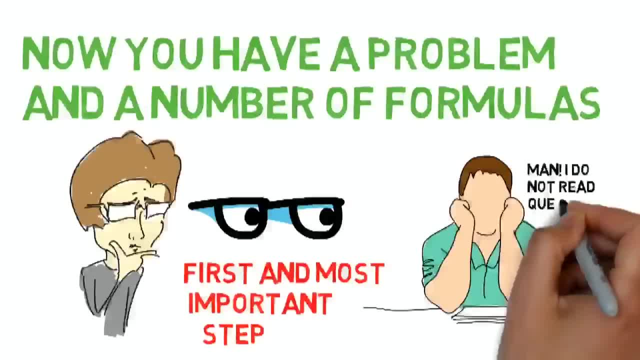 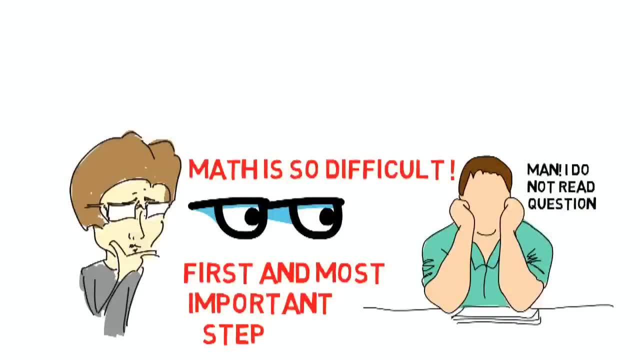 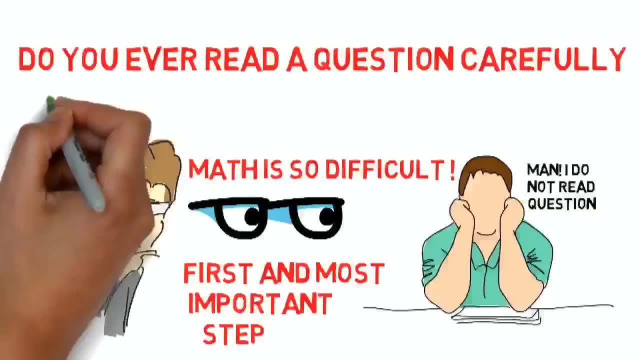 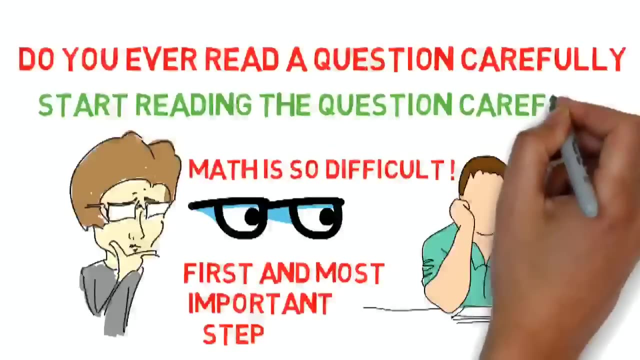 no, math is so difficult for me. ask yourself, do you ever read a math question carefully, ever without starting to solve the problem? if so, first read the question and then you will know that formula automatically which is going to be used in that problem, because you have a list of particular. 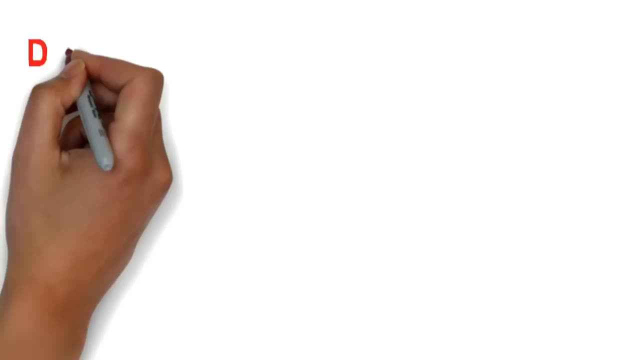 formulas which are going to be used in that chapter. then do not suddenly start solving the problem. first think in your mind: how will i get to the problem? i have an answer. first, answer the answer correctly, not the answer which is small. increase my progress and listen carefully. if 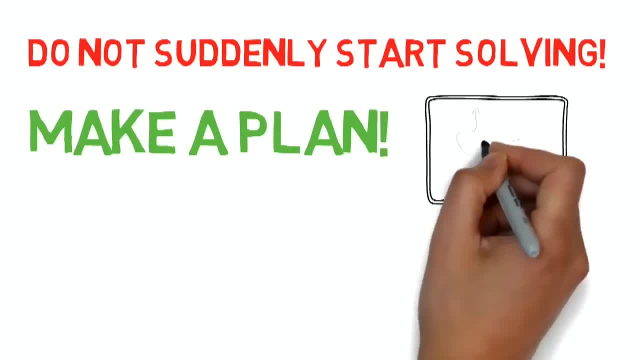 not small things can be done. you will automobile start by getting to the solution. first, use the. put a fingers here and do not reflect on the numbers. hold a bunch of small notes and draw them. from these value in the question to the one value of the answer, i have to use the formula which i: 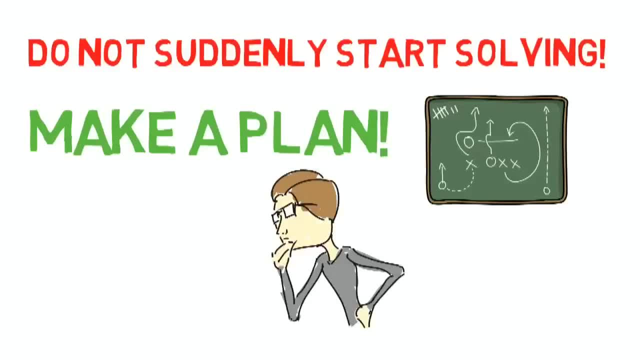 have what to do. think, use your mind. this will make math super interesting. it is like solving a puzzle game. you have given a puzzle and you have some patterns, some formulas to solve the problem and you have to get to the answer, to the goal. so how will you solve the problem? think in. 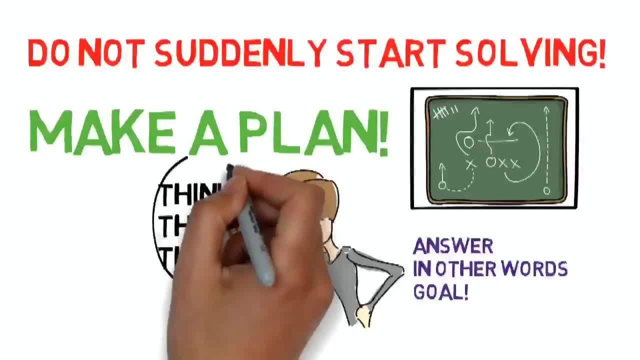 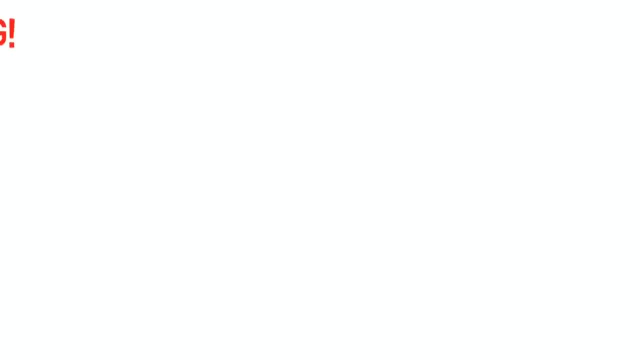 your mind what i have to do, what i have to change the values. i have to change these numbers to this and then apply this formula, make it super interesting in your mind and then start solving the problem. let's say, you got a wrong answer. you tried again, you again got the wrong answer. 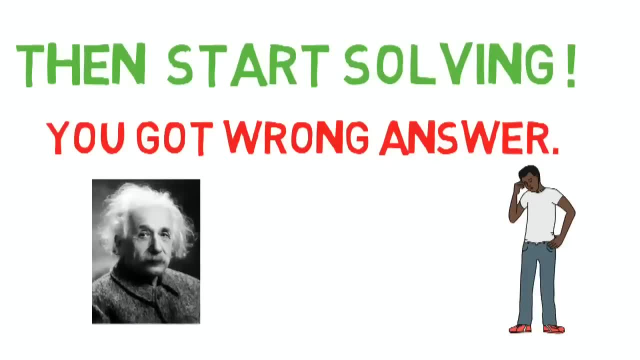 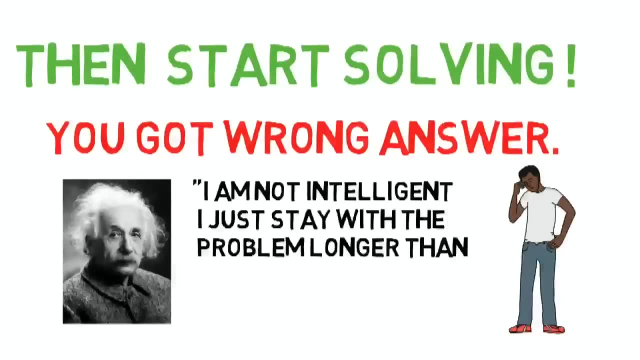 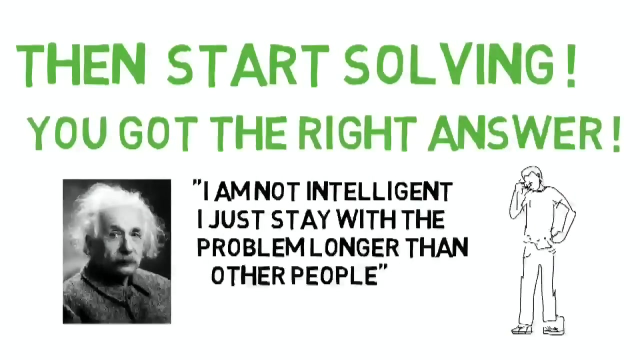 no problem, you have to try again always remember. einstein said: i am not intelligent, i just stay with the problem longer than other people. so the longer you will be with the problem, the more chances that you will solve the problem correctly and at last you will get the right answer. yes, you just solved a math. 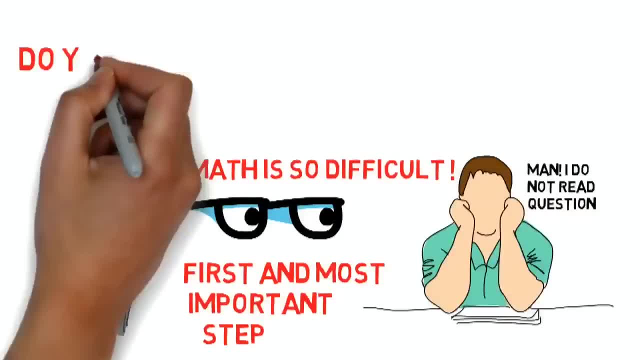 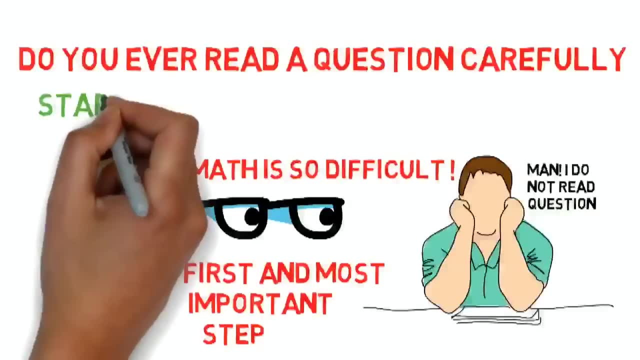 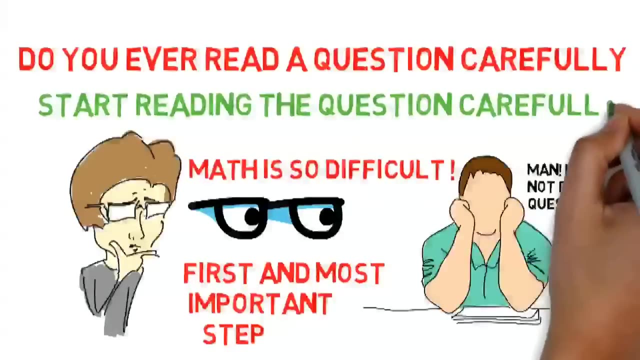 difficult for me ask yourself: do you ever read a math question carefully, ever without starting to solve the problem? if so, first read the question and then you will know that formula automatically which is going to be used in that problem, because you have a list of particular formulas which are going to. 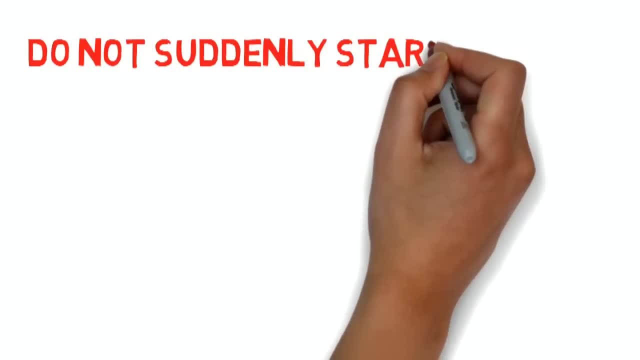 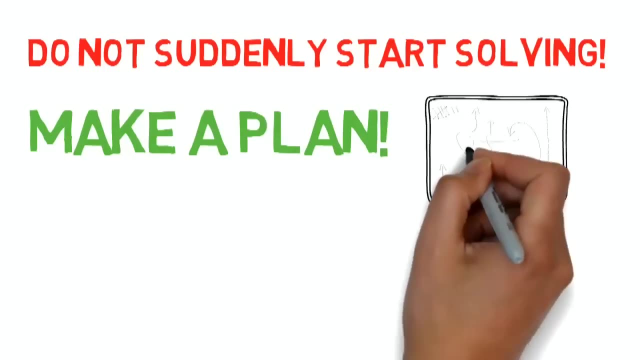 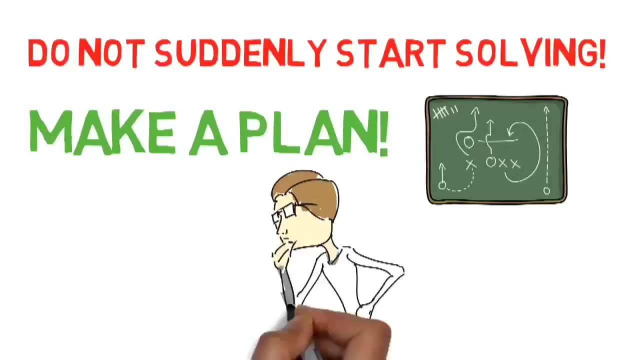 be used in that chapter. then do not suddenly start solving the problem. first think in your mind: how will I get from these value in the question to the one value of the answer? I have to use the formula which I have. what to do? think, use your mind. this will make math super interesting. it is like solving a puzzle. 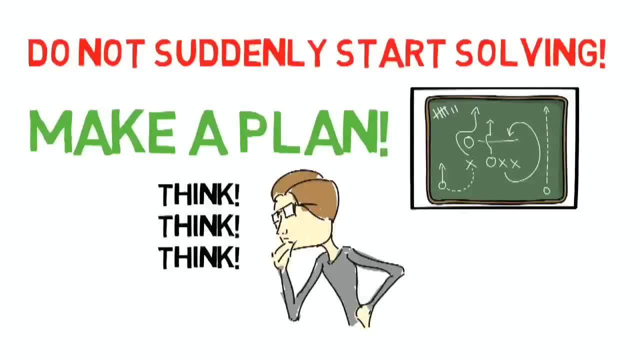 game. you have given a puzzle and you have some patterns, some formulas to solve the problem and you have to get to the answer, to the goal. so how will you solve the problem? think in your mind what I have to do, what I have to change the values I have. 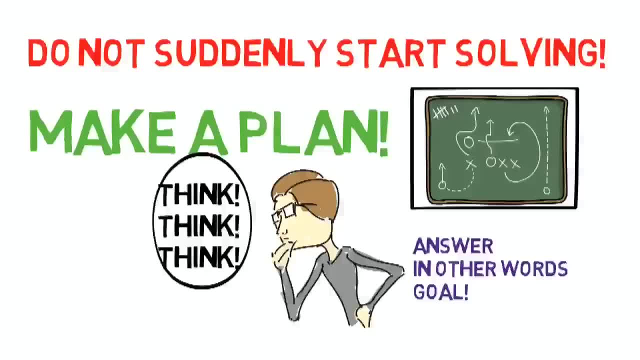 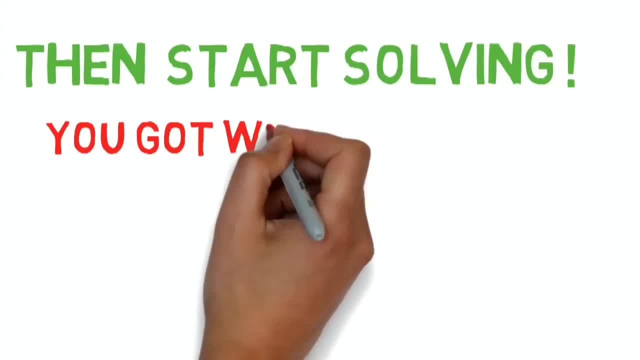 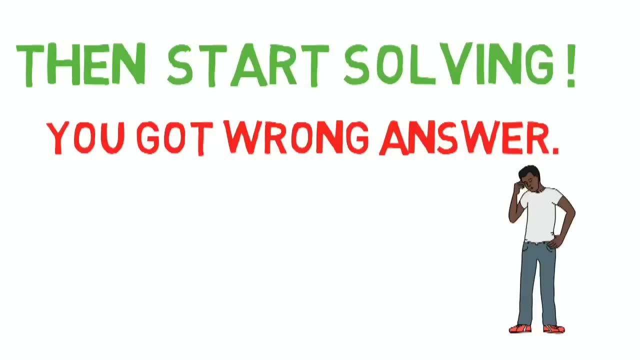 to change these numbers to this and then apply this formula, make it super interesting in your mind and then start solving the problem. let's say, you got a wrong answer. you tried again. you again got the wrong answer. no problem, you have to try again. always remember Einstein said: I am NOT intelligent, I just 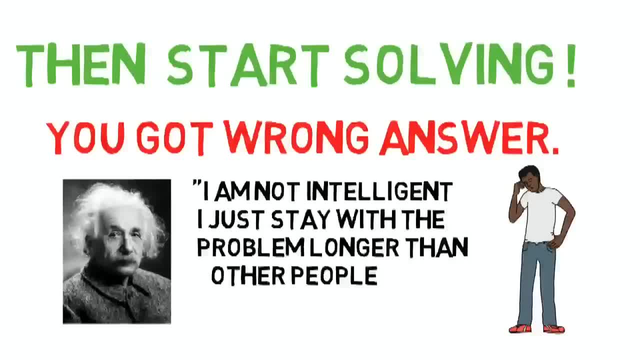 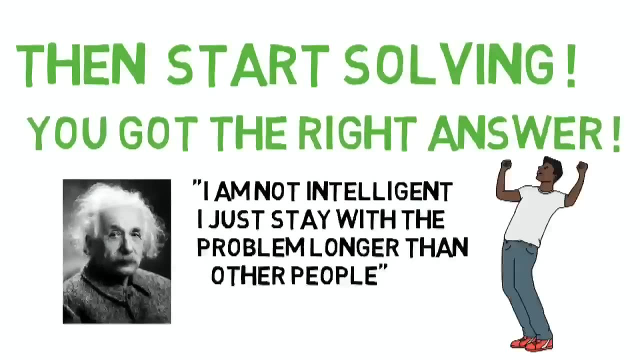 stay with the problem longer than other people. so the longer you will be with the problem, the more chance is that you will solve the problem correctly and at last you will get the right answer. yes, you just solved a math problem on your own without any help book, congrats. now you have to open a help book and see if 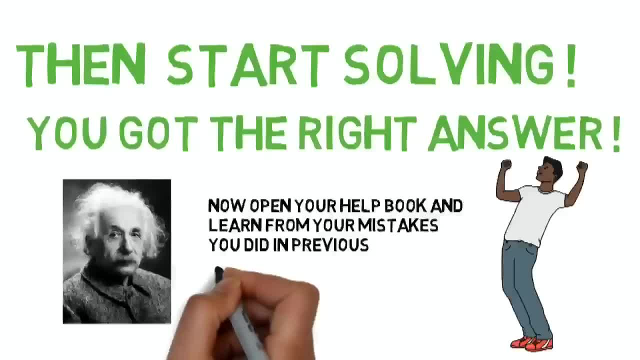 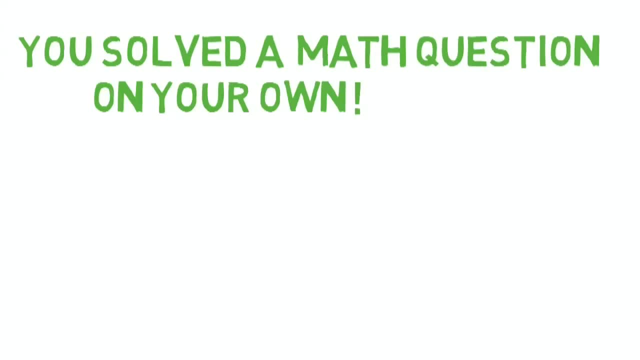 your solution is right and learn from your mistakes. you did in the previous question. basically, this is learning: learning from your mistakes. this will make your brain more sharper. now you just hold a math problem on your own, but do you think you did? you made billions of connections in your mind. you are using the trial and 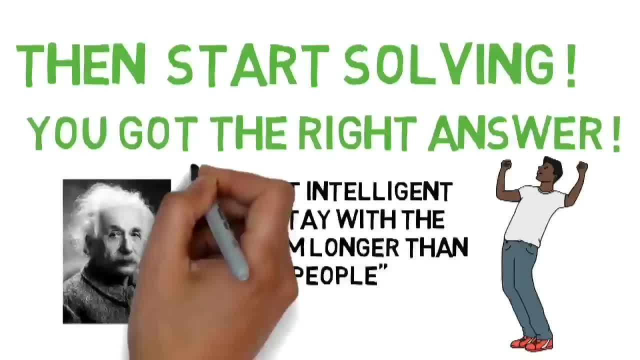 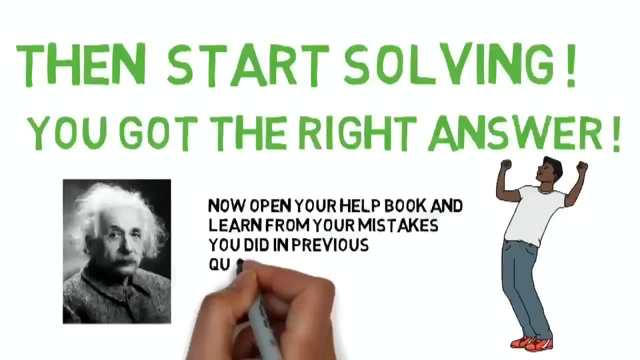 problem on your own without any help book- congrats. now you have to open a help book and see if your solution is right and learn from your mistakes you did in the previous question. basically, this is what i hope you learned, and you learned something in this video that will happen and also the next. 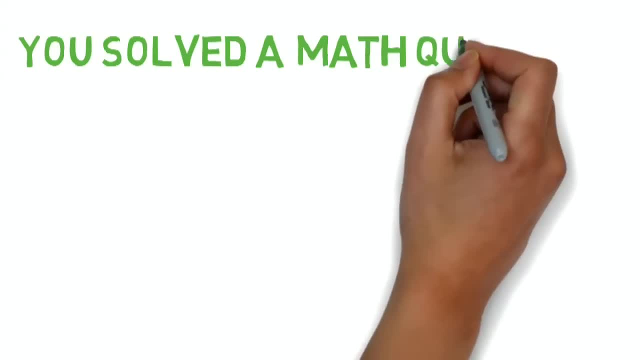 question that you learn is: this time around, you will learn something you should have brought you- able to run this game without using any particular formula this time- and that is learning from your mistakes. this will make your brain more sharper now. you just called a math problem on. 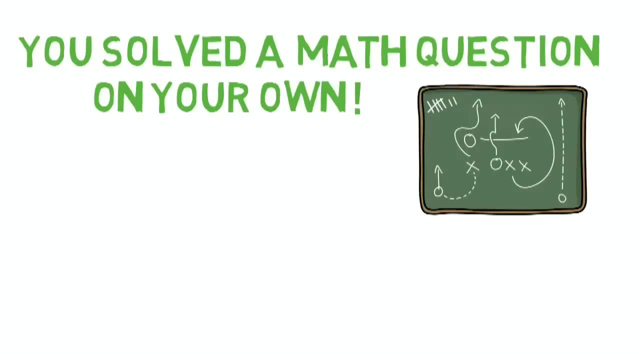 your own. what do you think you did? you made billions of connections in your mind. you are using a trial and error method and constantly learning from your tries, and by this you will start memorizing formulas easily, because you will take up a formula and apply that in your question and this. 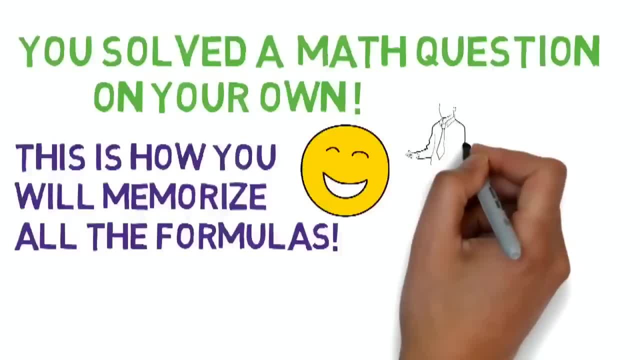 automatically appear in your book. so for this website you can fill out a formula that you can use your brain well and you have good honor to use this knowledge to answer a lot of questions and if you automatically memorizes formulas. I tried this and all the math formulas just stamped in my mind. 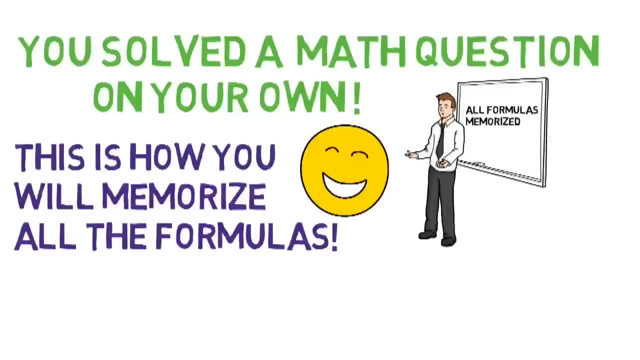 If you practice this, then you can solve any question in that chapter. Remember, Einstein said: Imagination is more powerful than knowledge. If you don't memorize formulas, no matter, But you should have that mind which is required to solve that problem, A mind which has full of. 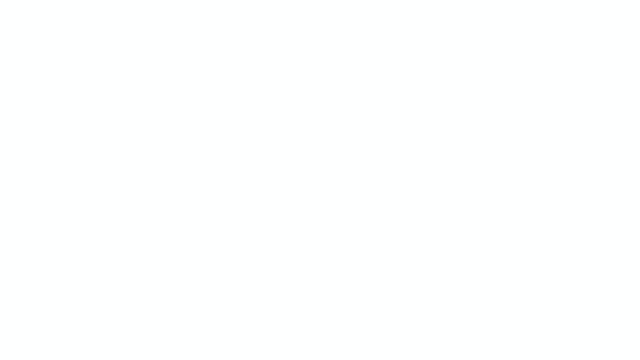 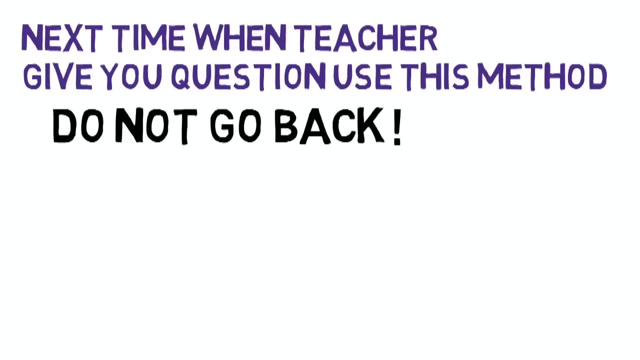 Imagination that how you can get to the answer. So next time when your teacher gives you a homework of a question, Try to use this method. This method will make math super interesting for you And it will be like playing a video game. And please do not go back to what you were when you opened this video. 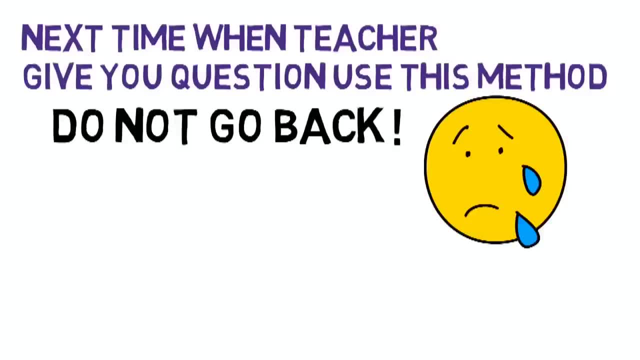 Because there is no other way to solve math more easily than this. There are lots of other videos which tell how to solve math easily, How to become a genius, etc. etc. But there is no other way. They will give you tips, routines, etc. 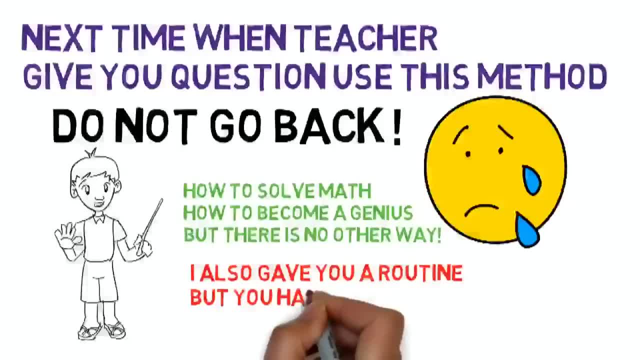 Like: I also gave you a routine, But you have to stick with something, Something in this video or in any other video. Okay, so take a simple thing and stick with it, Like if you say: I do not want to do all this from tomorrow. 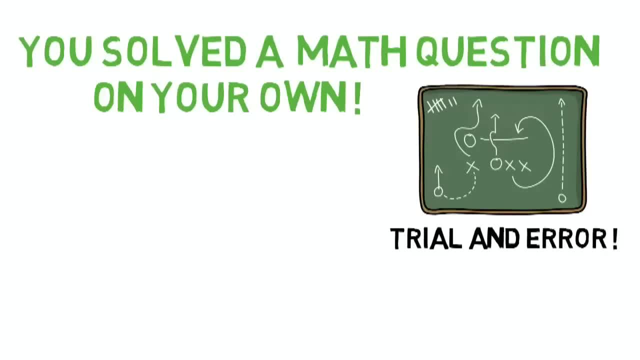 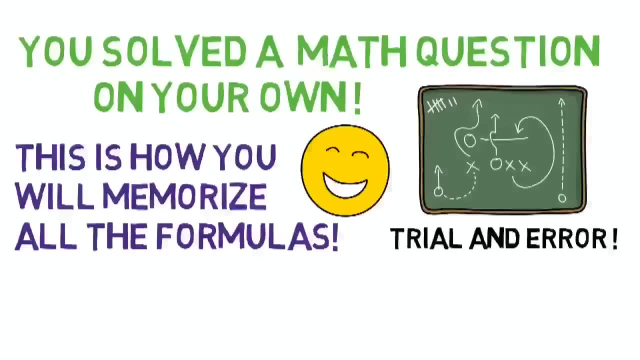 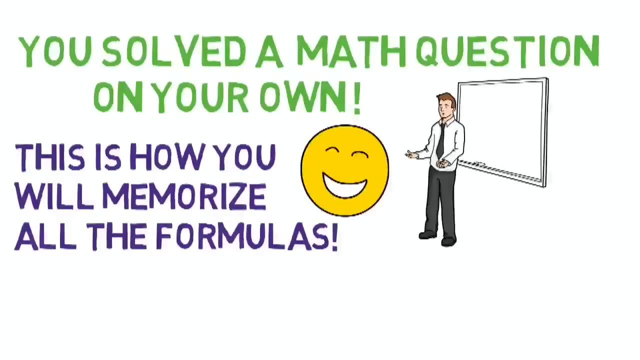 error method and constantly learning from your tries, and by this you will start memorizing formulas easily, because you will take up a formula and apply that in your question and this automatically memorizes formulas. I tried this and all the math formulas just stamp in my mind. if you practice this, then you can solve any. 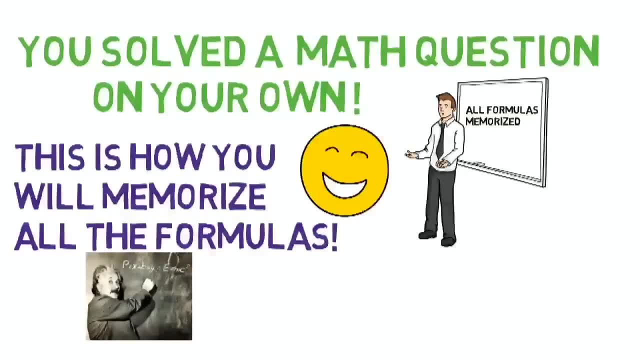 question in that chapter. remember, Einstein said: imagination is more powerful than knowledge. if you don't memorize formulas, no matter, but you should have that mind which is required to solve the problem. a mind which has full of imagination that will solve the problem. a mind which has full of imagination that will solve the problem. 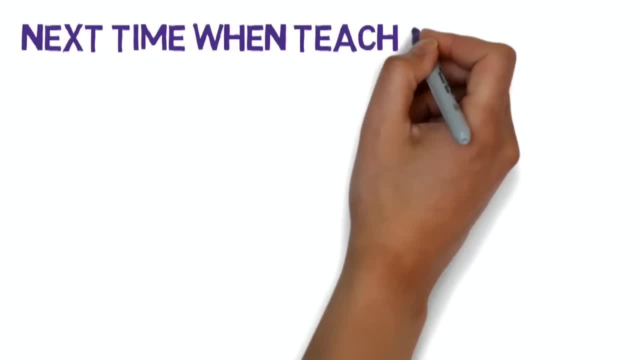 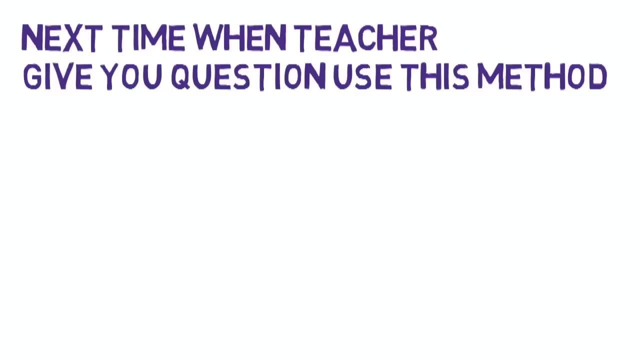 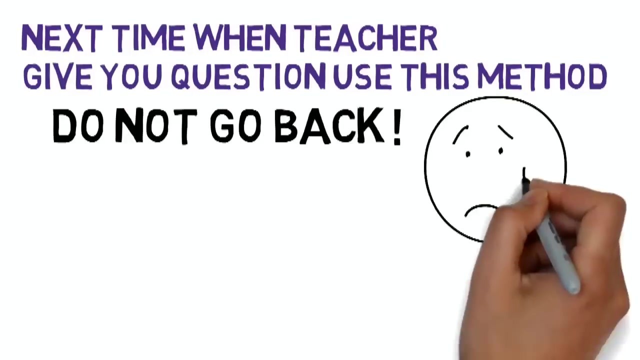 how you can get to the answer. so next time when your teacher give you a homework of a question, try to use this method. this method will make math super interesting for you and it will be like playing a video game. and please do not go back to what you were when you open this video, because 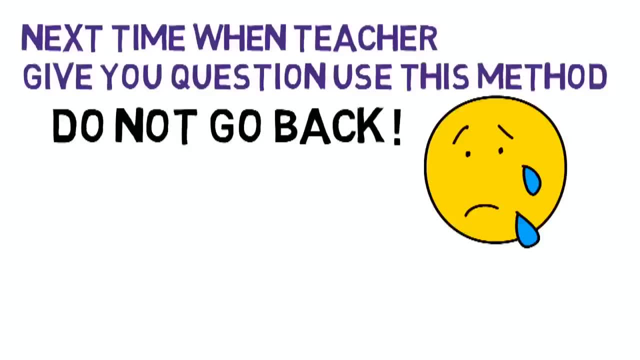 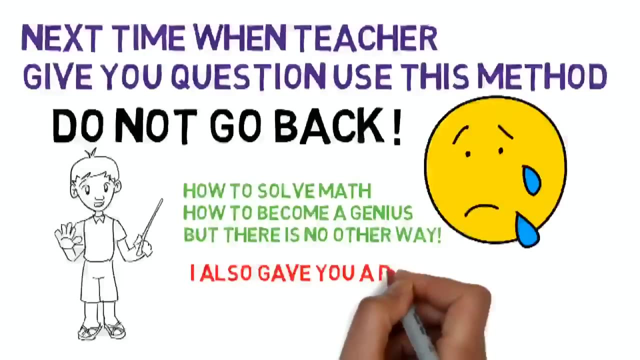 there is no other way to solve math more easily than this. there are lots of other videos which tell how to solve math easily, how to become a genius, etc. etc. but there is no other way. they will give you tips, routines etc, like i also gave you a routine, but you have to stick with something. 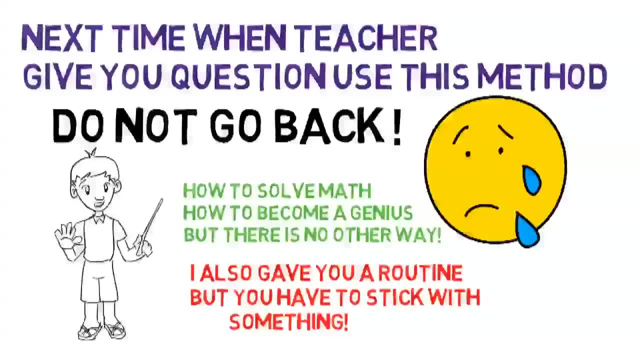 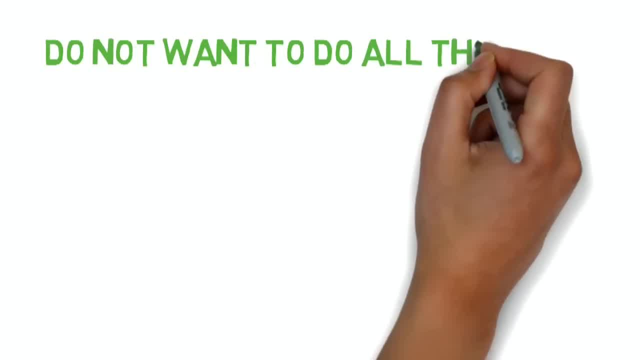 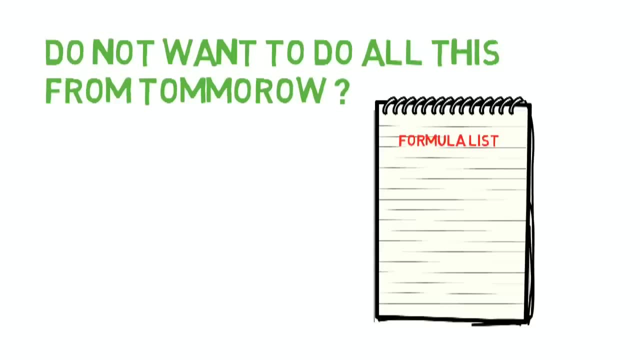 something in this video or in any other video. okay, so take a simple thing and stick with it, like if you say i do not want to do all this from tomorrow, just do a simple thing like making a list of all the formulas in your chapter. this will change something and you will start growing. so slow and steady wins. 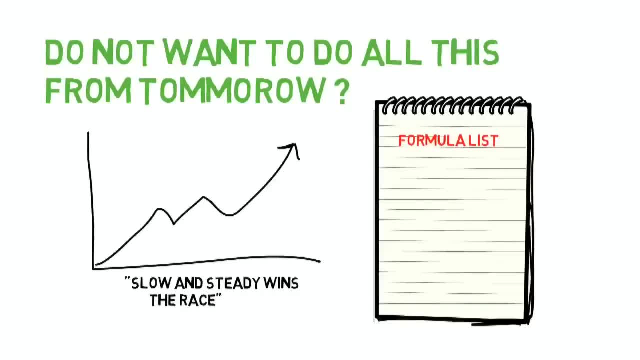 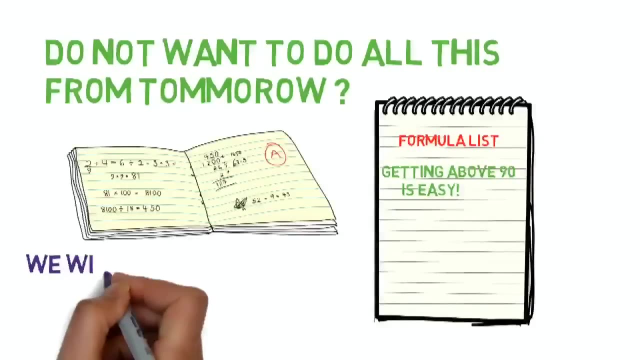 the race. now you know the way, the single key to success in mathematics. if you follow this, getting above 90 is a piece of cake for you. now let's get something practical. we will take a universal math problem of seven standard so that everybody can understand it, and we'll apply this method to 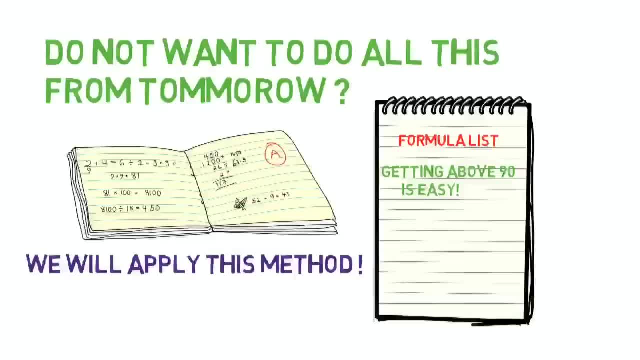 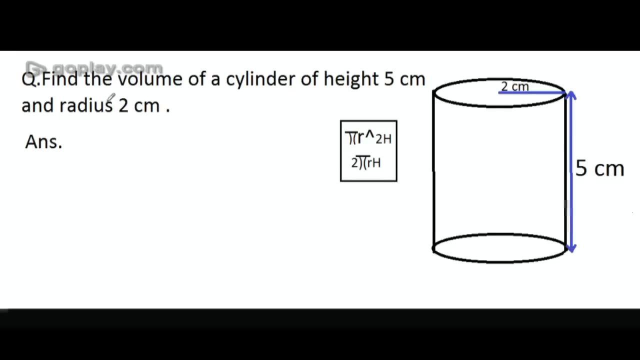 solve that problem. if you are a high standard student, then see how i will solve that problem and apply the same method in your math problem. this will clear this concept to you more. so let's begin. take a look at this simple math question. this is a seven standard. 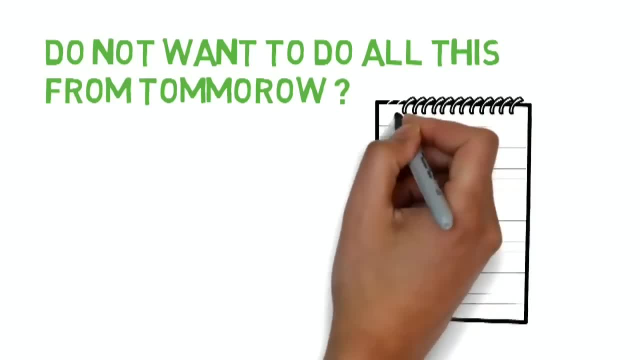 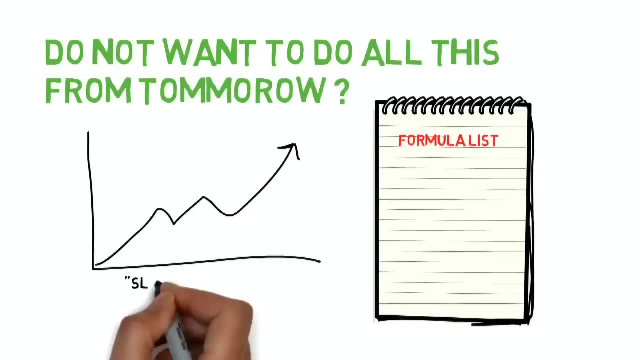 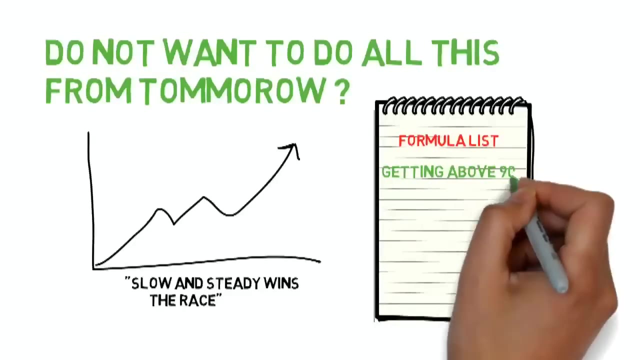 Just do a simple thing like making a list of all the formulas in your chapter. This will change Something and you will start growing so slow and study wins the race. now You know the way- the single key to success in mathematics. If you follow this, getting above 90 is a piece of cake for you. Now let's get something practical. 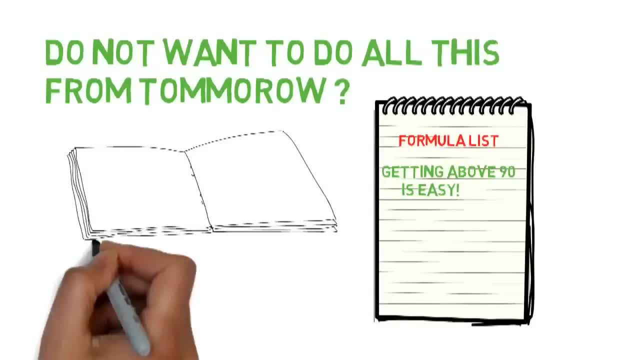 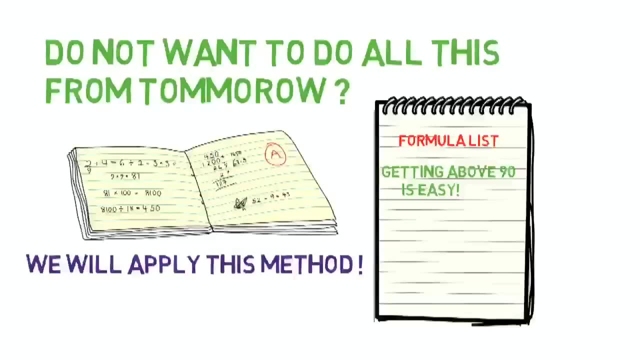 we will take a universal math problem of seven standard so that everybody can understand it and Will apply this method to solve that problem. If you are a high standard student, then see how I will solve that problem And apply the same method in your math problem. This will clear this concept to you more. So let's begin. 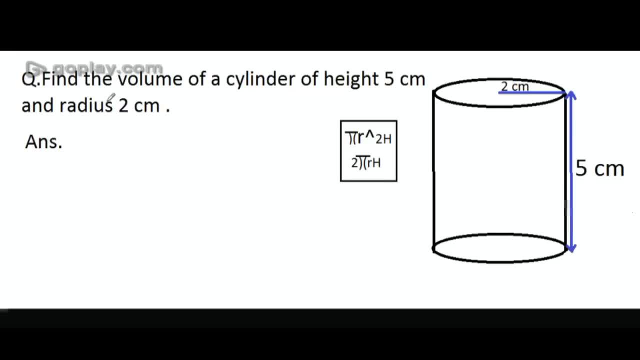 Take a look at this simple math question. This is a seven standard math question. I took this question so that everybody can understand the mindset better. in this question You have asked to find the volume of the cylinder of height 5 centimeters and radius 2 centimeters. 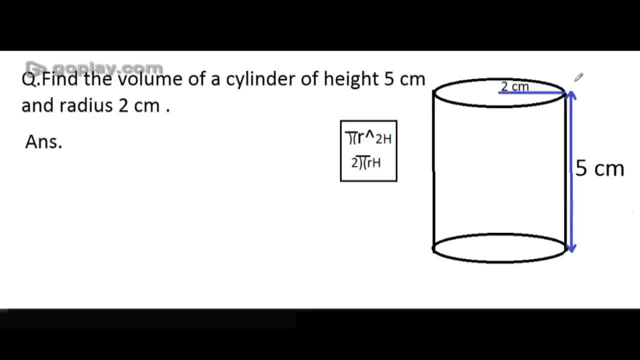 This is a cylinder of height 5 centimeters and radius 2 centimeters for high standard students. Just assume this as a demonstration of that mindset. I will apply that mindset in this question to find the answer. Like say, we have a chapter in which we can find two types of function. 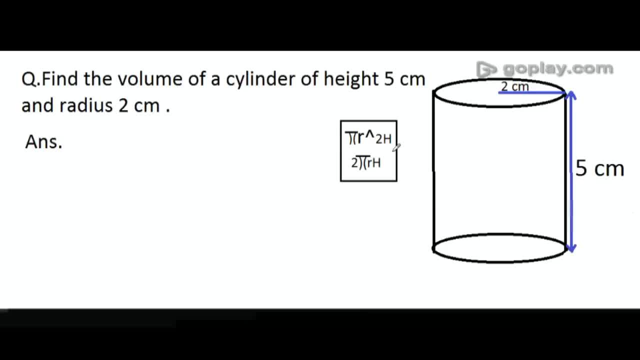 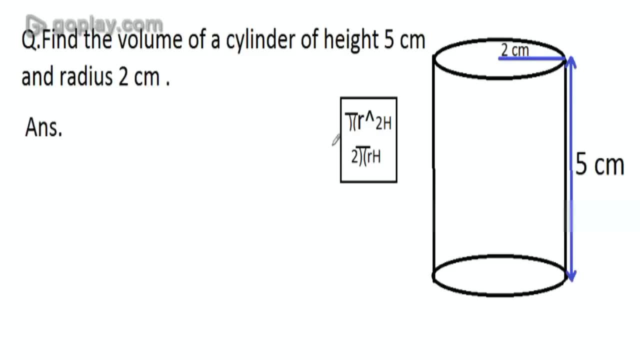 First is the volume of the sling and setting is the surface area of cylinder. and we are new to all this and we don't Know which formula is of volume and which formula is of surface area of cylinder or cylinder ideal formula is of surface area. so assume that this is happening and now we will apply the 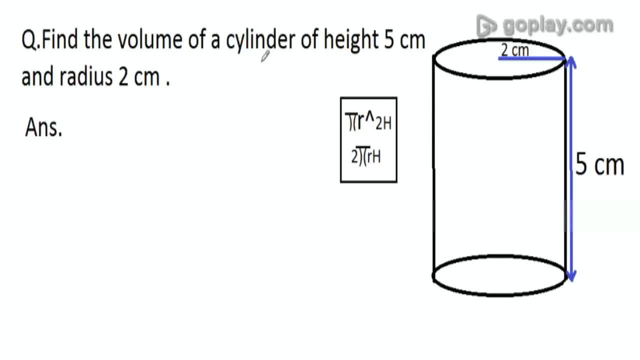 method to solve that problem. so first step is to read the problem carefully. in this problem we have to find the volume of cylinder of height 5 cm and radius 2 cm. for high standard students they will say that, oh, this question is super easy. this is of volume formula. we 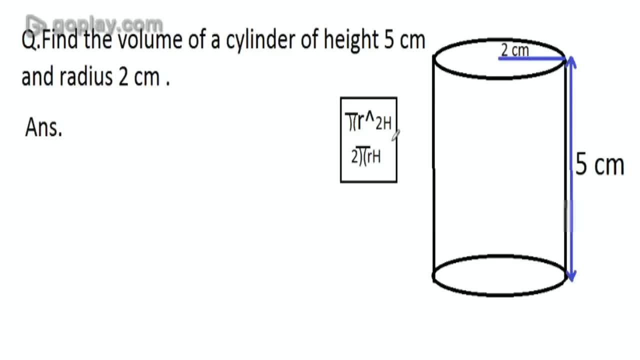 have to just chunk in these values and find the answer. but no, this is just a demonstration. take it as a demonstration and use the same method in your difficult questions. so we have these two values: first is height and second is radius of cylinder. now let us write first what is the radius of cylinder? radius of cylinder. 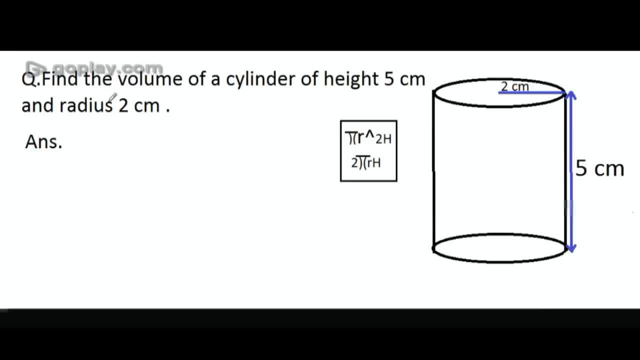 math question. i took this question so that everybody can understand the mindset better. in this question you have asked to find the volume of the cylinder of height 5 centimeters and radius 2 cm. This is a cylinder of height 5 cm and radius 2 cm For high standard students just. 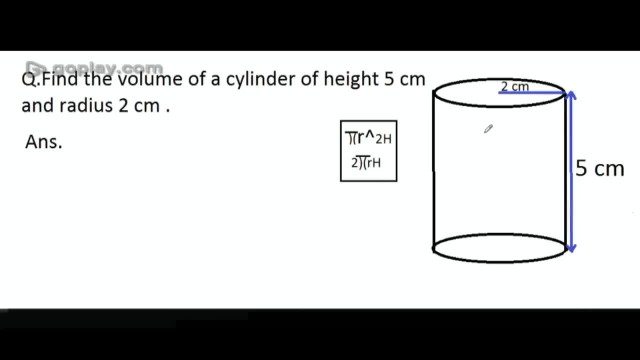 assume this as a demonstration of that mindset. I will apply that mindset in this question to find the answer. Let's say we have a chapter in which we can find two types of questions. First is the volume of the cylinder and second is the surface area of cylinder. And we are: 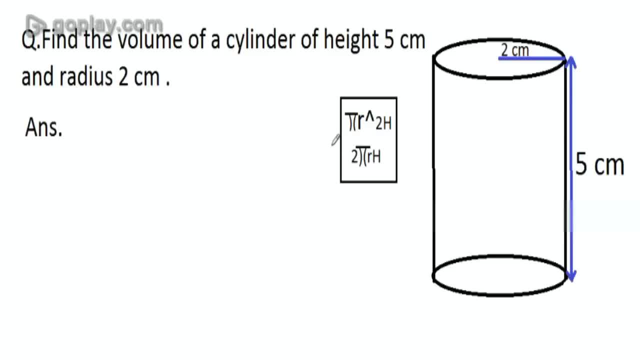 new to all this, and we don't know which formula is of volume and which formula is of surface area. So assume that this is happening and now we will apply the method to solve that problem. So first step is to read the problem carefully. In this problem we have to find the volume of. 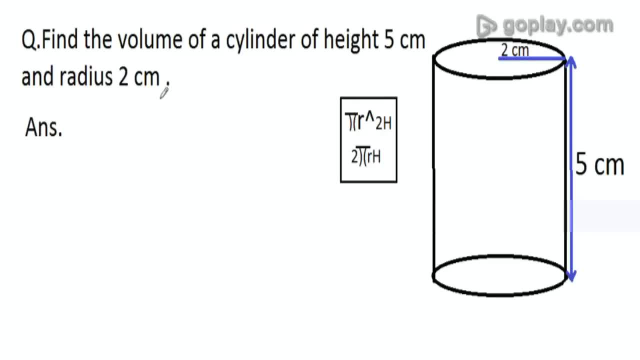 cylinder of height 5 cm and radius 2 cm For high standard students. they will say that oh, this question is super easy. this is of volume formula. We have to just chunk in these values and find the answer. But no, this is just a demonstration. 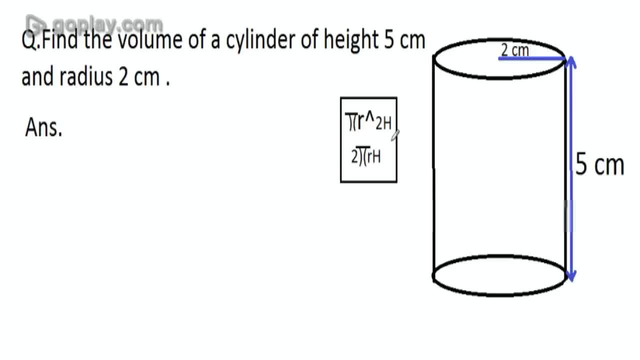 Take it as a demonstration and use the same method in your difficult questions. So we have these two values. First is height and second is radius of cylinder. Now let us write first what is the radius of cylinder. Radius of cylinder is equal to 2 cm and height of cylinder is equal to 5 cm. So we have these two values. 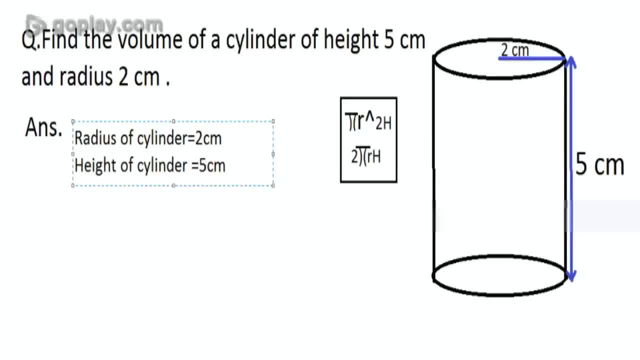 And we have to get from these two values to the one value of the volume. How do we get there? We have to use one formula, one formula of the volume. what do we do? what we have to do? so, first we have to know which formula is of volume, and 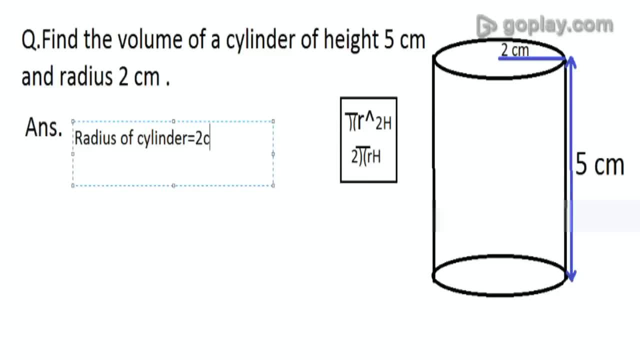 is 2 cm and height of slender is equal to 5 cm. so we have these two values and we have to get from these two values to the one value of the volume. how do we get there? we have to use one formula, one formula of the volume. 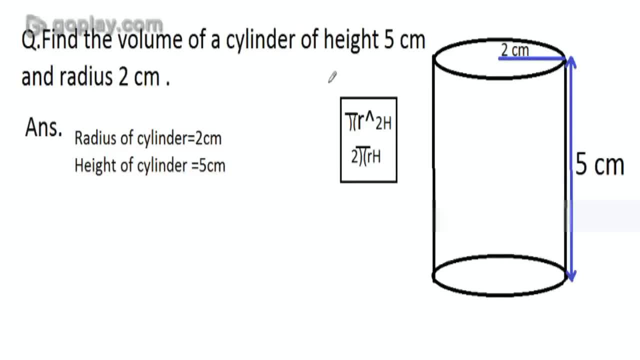 what do we do? what we have to do? so first we have to know which formula is of volume and which formula is of surface area. so how do we know that? see this: what is the area of circle? that means all this. what is the area of circle that is pi? r square right. so we have the area of circle, this: 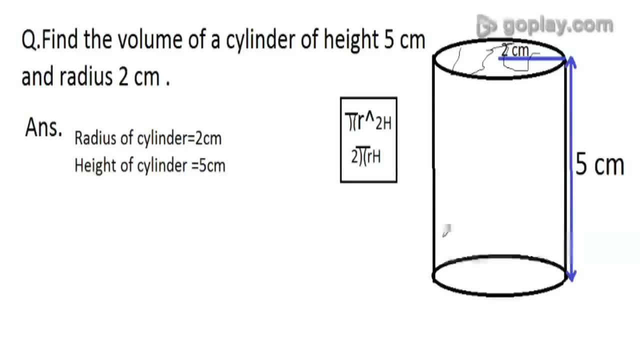 and if we multiply it by the height, which is this, then we will have a circle stacked on each other to five centimeters high and then we will have the volume. so we know that this formula is of volume and for surface area, tell me the parameter of circle, that is, two pi r right. and if we have 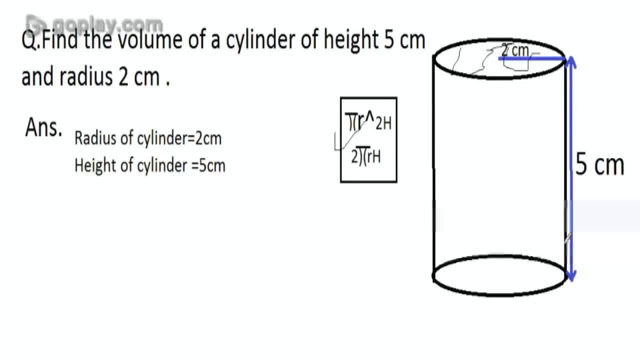 hollow circles stacked on each other to five centimeter. then we will have the surface area of cylinder right. so we know that volume of cylinder is this and we will apply this in the our question. so volume of cylinder is equal to, so the volume of cylinder, which is this formula, and we will 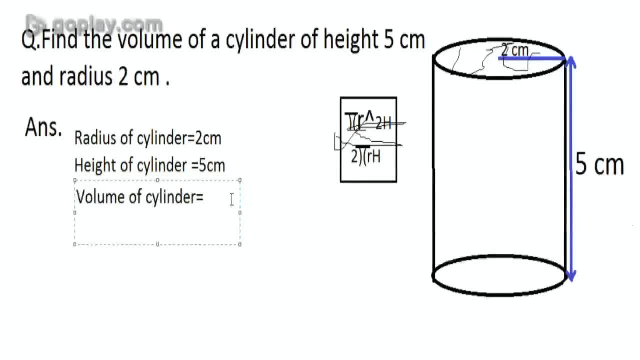 apply that in our question, that is, pi r square h. so we first have to chunk in the values. okay, so let's chunk in the values: pi is 3.14 multiplied by r square, which is 2, and 2 square is equal to 4 multiplied by h, which is height, which is 5 centimeter, and now this is equal. 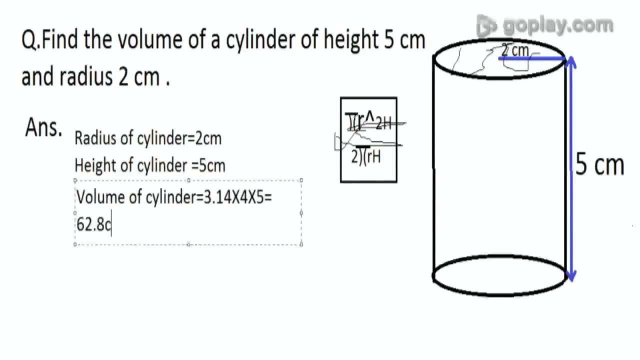 to 62.8 centimeters cubed. never forget to add the unit after the transformation. we are going to talk about the unit now. let's start class two. remember the value in math. This is also very important tip for math. So we just read the question. 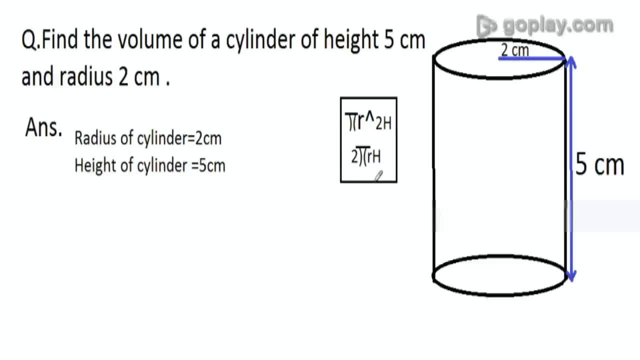 which formula is of surface area. so how do we know that? see this: what is the area of circle? that means all this. what is the area of circle? that is pi, r, square, right. so we have the area of circle, this, and if we multiply it by the height, which is this, then we will have a circle. 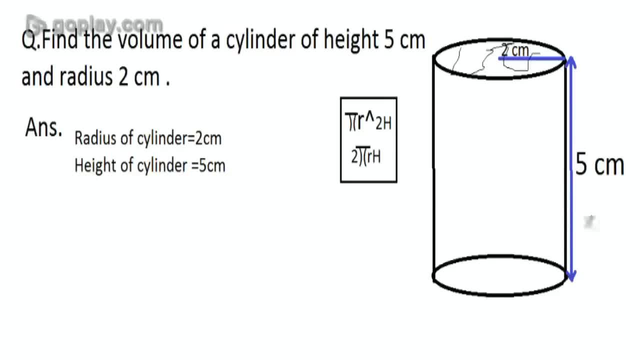 stacked on each other to 5 centimeter height, and then we will have the volume. so we know that this formula is of volume and for surface area. tell me the parameter of circle, that is, 2, phi, r, right. and if we have hollow circles stacked on each other to 5 centimeter, then we will have the 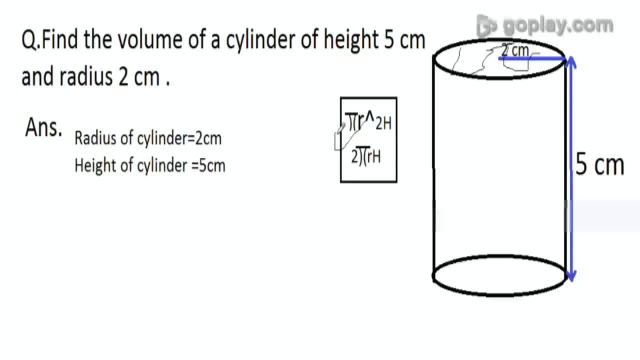 surface area of cylinder. so we know that volume of cylinder is this and we will apply this in our question. so volume of cylinder is equal to. so the volume of cylinder, which is this formula and we will apply that in our question. that is pi r square h. so we first have to chunk in. 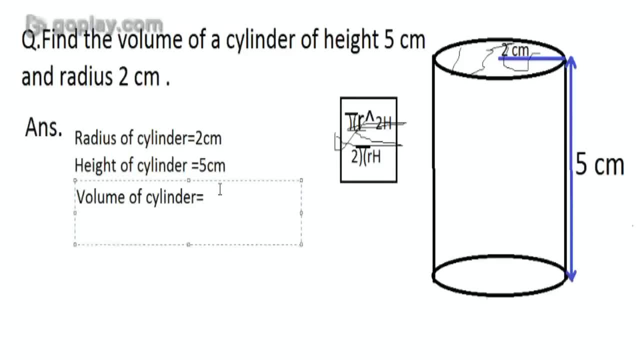 the values. okay, so let's chunk in the values. pi is 3.14 multiply by r square, which is 2, and 2 square is equal to 4, multiply by h, which is height, which is 5 centimeter, and now this is equal to 62.8 centimeter cube, never forget to add the unit. 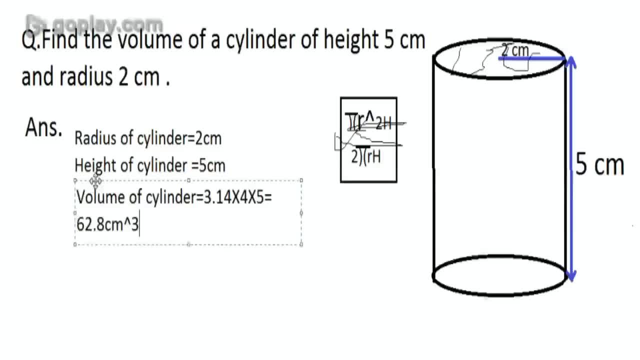 after the value in math. this is also very important tip for math. so we just read the question carefully, knew which formula is to be applied, first thought what we have to do and then did it and found the answer. and this is how you should always solve a math question. 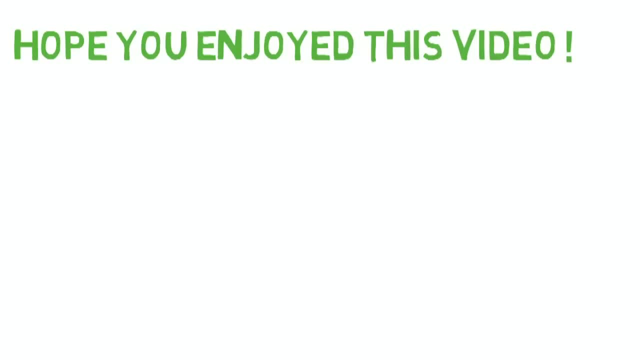 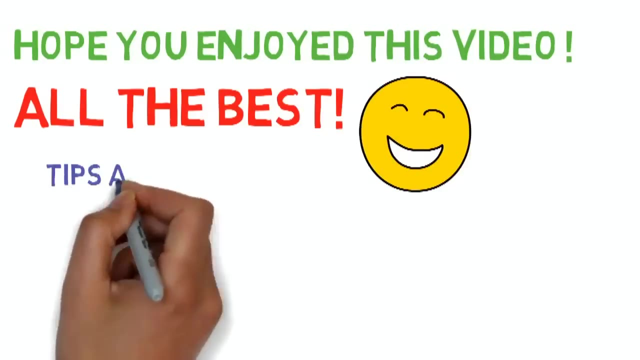 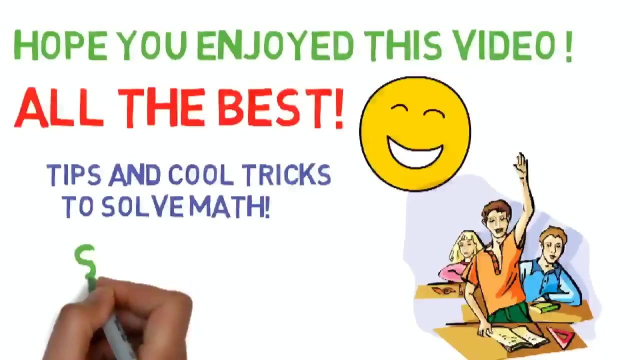 hope you enjoyed this video. i wish you all the very best for your further math studies. in my next video, i will share some amazing tips and some cool tricks which will definitely help you to make math more easy. so subscribe this channel to get notified for my next video. and finally, thanks for watching.